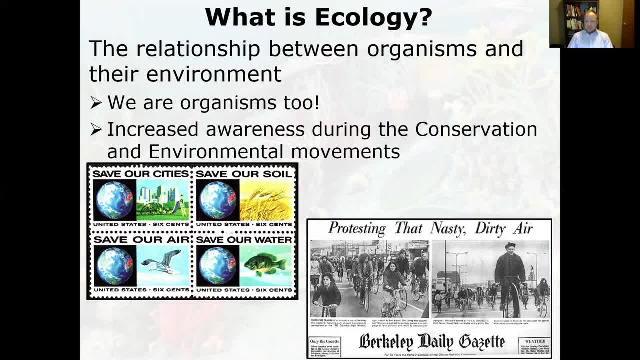 their environment, And it's a two-way street, So it's how the environment affects the organisms, but also how the organisms affect the environment. And remember that we humans- we are organisms as well, So we are part of this ecology And this really started increasing as a thing. 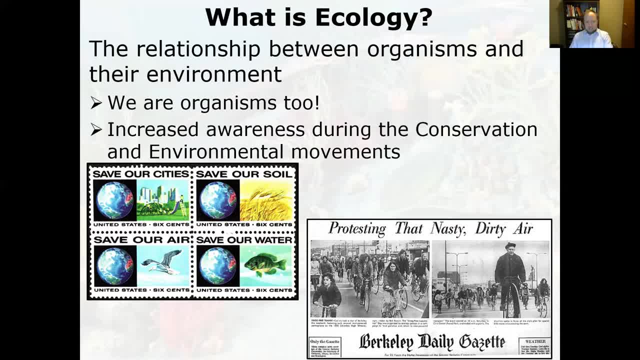 in the 1900s, with the conservation effort and the environmental movements. So sees things like this, So like: save our cities, save our soil, save our air, All these reports of like rivers catching on fire, not ideal. So fortunately we cleaned up a lot of that stuff, A lot of 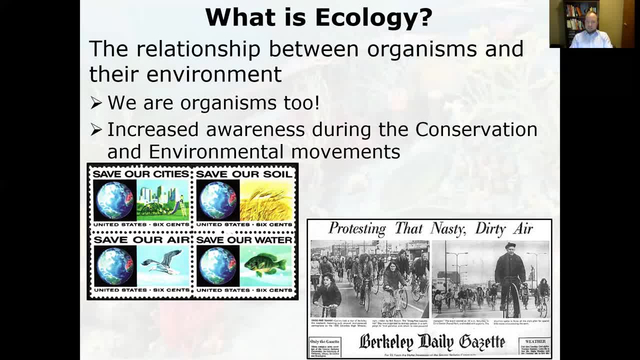 smog issues have been kind of alleviated. Obviously it's not where we'd like it to be, But ecology really came to the forefront with the environmental movement. A lot of college protests, especially like Berkeley, were kind of the centers for this. So young 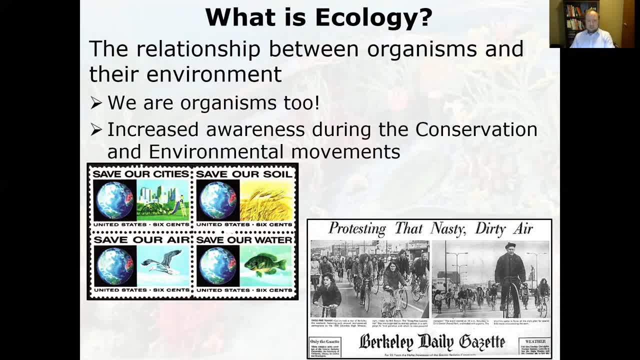 people really pushed this movement of becoming aware of basically how we as organisms are impacting our environment, And then obviously that impacts us back. If we pollute our environment, it affects us in ways as well. So that's ecology And obviously this is paleontology class. 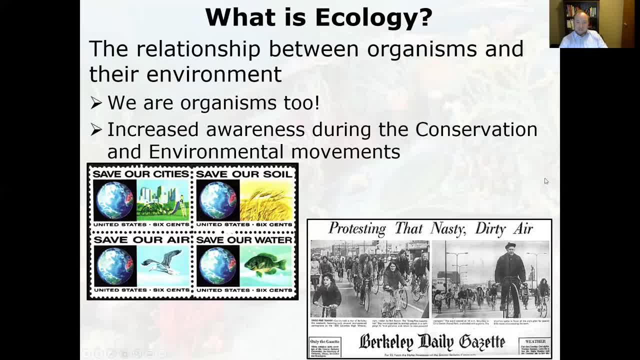 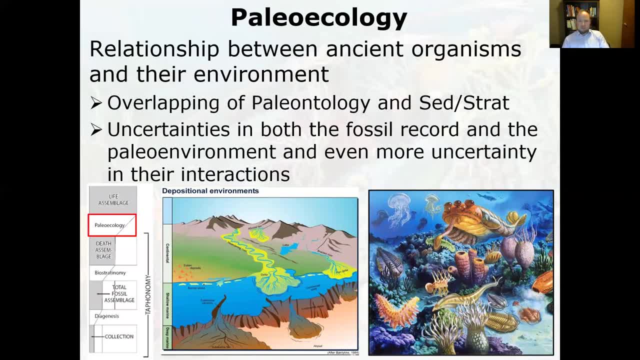 So we're going to talk about ecology in the past, Which is called paleoecology. So paleoecology, relationship between ancient organisms and their environment. It's really kind of where paleo- the stuff that we've been talking about. 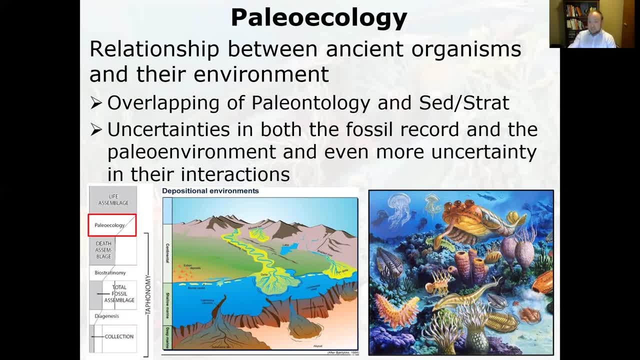 and said: strat, the stuff that we talked about, you know, last semester. it's really where these things kind of come together- So hopefully you remember this figure here from earlier in the course- Where we've got the life assemblage, the life community. This is what paleoecology is after. We're trying. 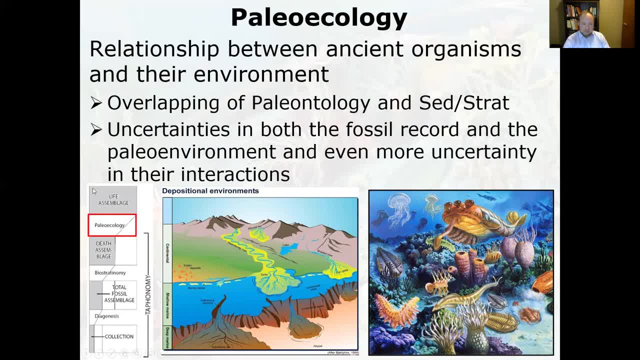 to kind of reassemble this life assemblage- And we're doing that from remember, not even actually the death assemblage, Because we don't actually even see the death assemblage, Because some of it doesn't make it into the fossil record Of the stuff that does make. 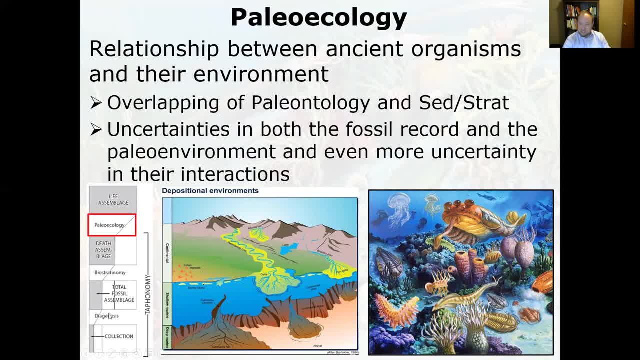 it into the fossil record. a lot of that is destroyed along the way, And even less of it is actually observed and collected. So we're trying to reconstruct this vibrant living community of diverse organisms from only what's recorded in the fossil record, This very small sliver. 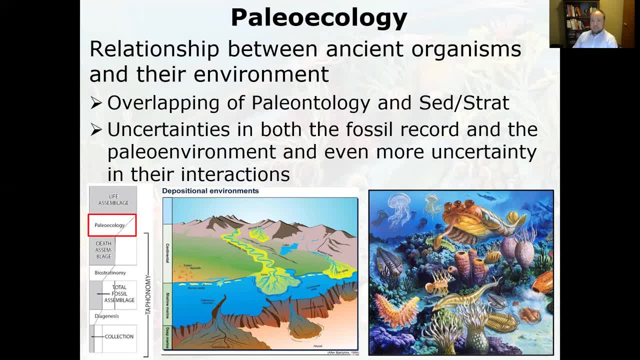 Obviously, that's a bit challenging. So take a look at this picture over here. Take a look at this. This is a Cambrian environment here, Reflecting organisms from the Burgess Shale. Take a look at some of those. But this is a very small. This is a very small, very small. 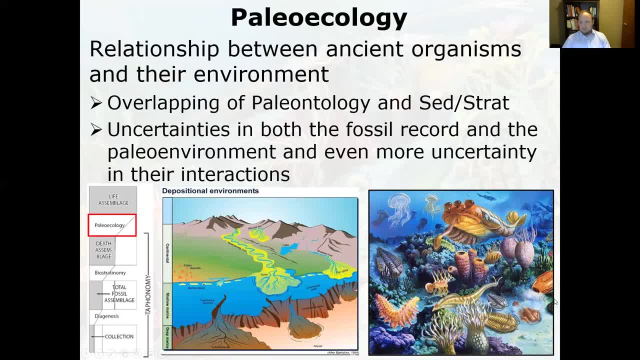 very small. If you look at some of the things here, You can see that there's a lot of the of those organisms there which ones are probably not going to be represented in the fossil record, so i'll give you a couple seconds to take a peek at that. look at all the different various critters. 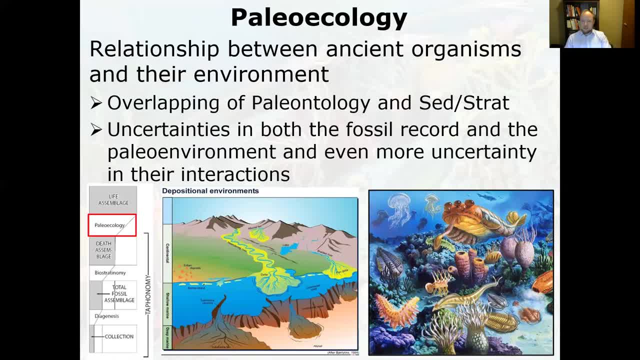 there. think about their structure, think about their morphology. what are they made out of? what's their life habit? how robust are they? so what do you think looking at that picture there? hmm, well, one thing that you probably thought about up here: these jellyfish they do not have. 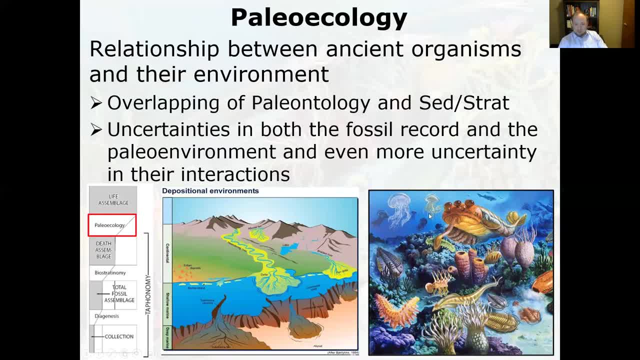 any hard parts. they're part of the community. they're probably a rather important part of the community. they will not make it into the fossil record. uh, these trilobites, trilobites, arthropods, remember they shed their exoskeletons. they may be actually over represented in the community because 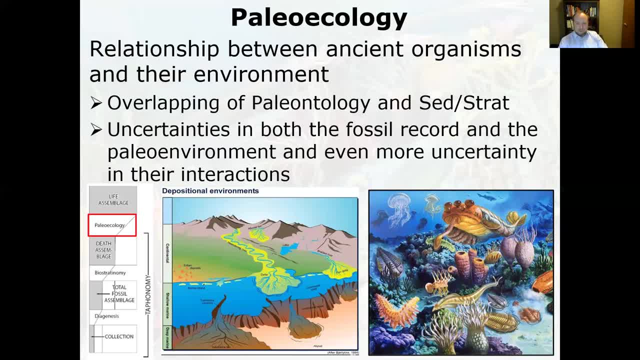 they have several different copies of themselves throughout their lifetime. sponges here, big hard parts, spicules- um, they'll probably be disaggregated into their parts, but they'll probably be represented. so there's a lot of different things that go into, uh, reconstructing this. you're trying to reconstruct this life assemblage from the. 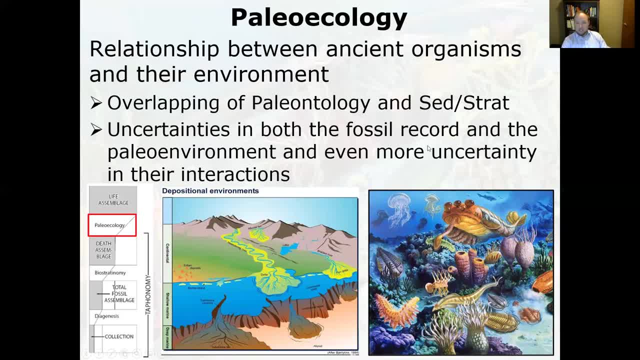 flawed fossil record and at the same time, we're trying to reconstruct the paleoenvironment. so for those of you that were in sedimentology stratigraphy last semester, we know the challenges that go into that. so, taking a look at our grain size, our grain texture, our 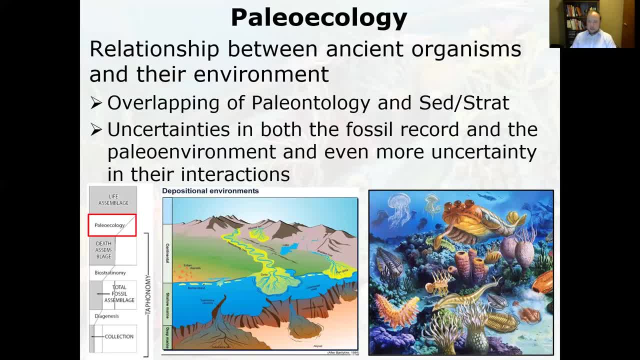 grain, shape, our sorting our sedimentary structures. uh, what environment was this? so let's walk. you walk up to a shell on an outcrop. uh, is this a ancient lagoon, a low energy, like back reef? is this deep in the middle of the ocean? or is this a deep in the middle of the ocean? or is this a deep in the? 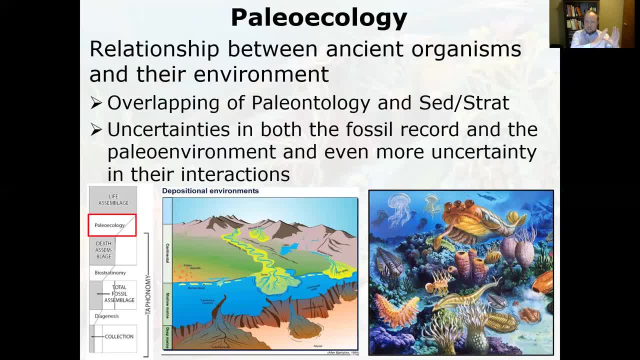 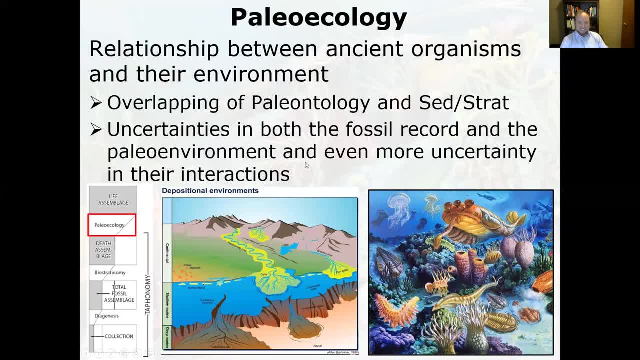 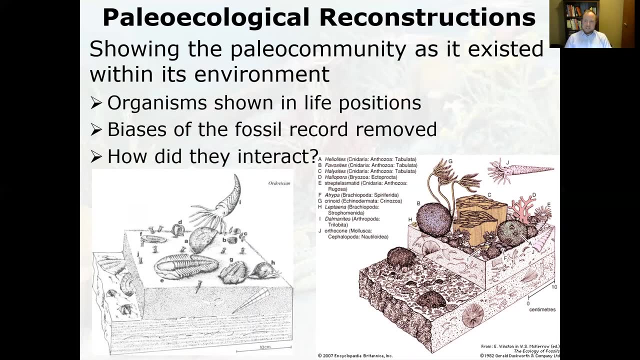 this is really paleoecology. it's where these two things are are coming together and, as you know, since we've discussed it, we're also trying to reconstruct the paleoecological reconstructions pretty dramatically. so probably one of the cooler things with paleoecology is that you get these paleoecological 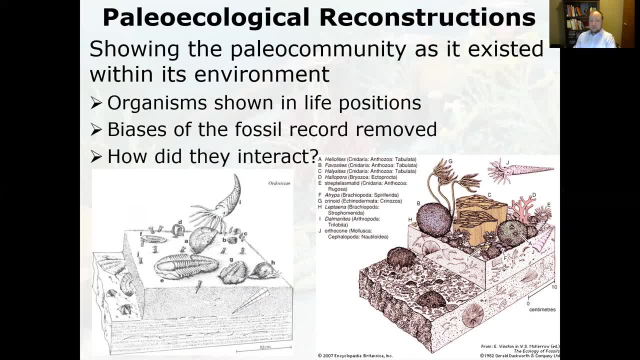 reconstructions. so there are these pretty pictures, very neat and very cool. they show the paleo community as it existed at the time, that it existed within its environment. so, for example, this over here view of what things might have looked like in the ordovician: we've got trilobites. we've got 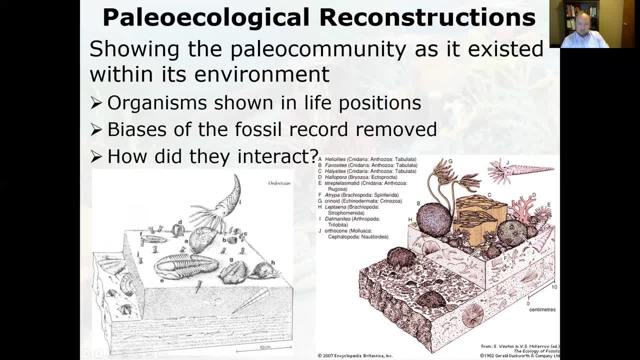 brachiopods. we've got a cephalopod predator and a straight shelled cephalopod, orthoconic cephalopod, swimming around chewing on all these things. we've got a gastropod: they're crawling around and these things are shown in their life positions, what they look like with their soft parts. 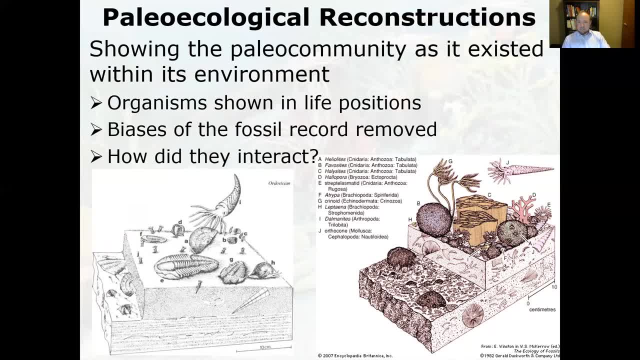 while they were living, an attempt to really just give you a look at what the what these things probably looked like. this one over here is a reconstruction of a silurian environment. so we've got our good friends here: phobosites, the tabulate coral, halicites, the chain coral. 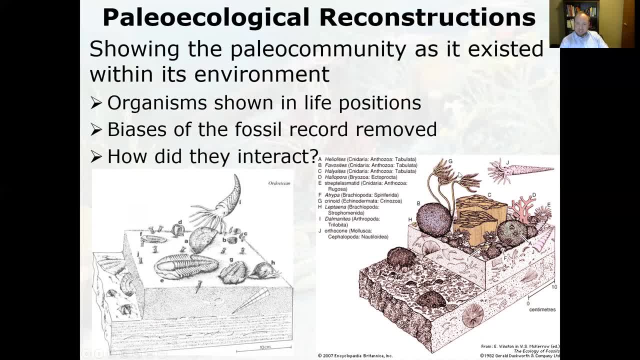 we've got some sea lilies, the crinoids, filter feeding in here. we usually see these as those fossil cheerios disaggregated completely, but on this reconstruction you see it's got that nice filter feeding calyx to kind of reach up into the water column and pull food out. we've still got these orthocoencephalopod. 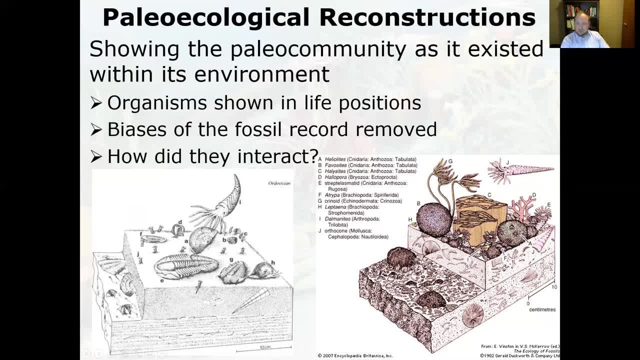 predators. we've got some of these branching bryozoans, very delicate, usually- broken up, but you can see everything's kind of been restored into its life position. what did this thing look like? with the biases of a fossil record removed, all of the biases of the soft? 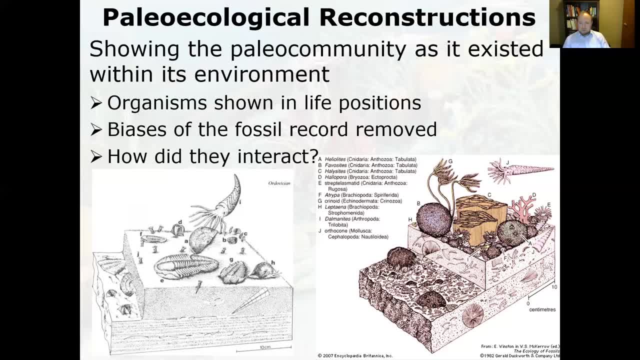 hearts, parts versus hard parts, the taphonomic processes- all that's been removed to kind of reconstruct what this environment looked like. and the other thing that we have to ask ourselves really is: okay, we've reassembled this living community, this, this life assemblage. how did they interact with each other? 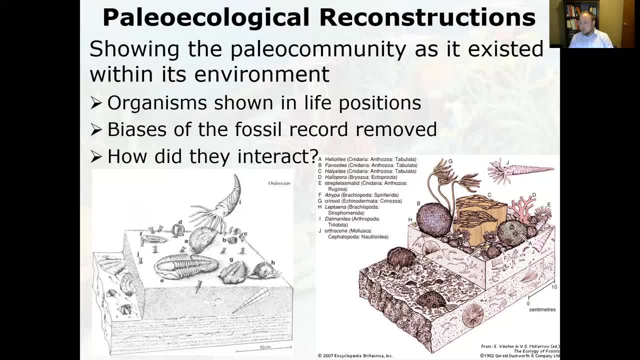 what was going on, who was chasing who, who was digging around in the soil, who was swimming in the water column, what were these critters doing when they were alive and what was going on with their lives. so let's take a look at these pictures real quick and remember we're trying to remove. 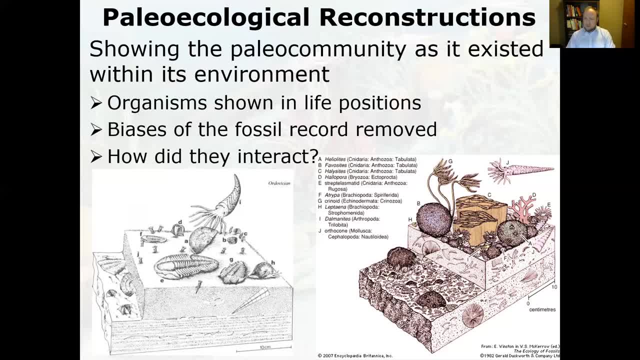 the biases of the fossil record here. what do you notice about this? do you think they did a good job with that? these are sort of older reconstructions from like the 70s and 80s, uh, sort of at the forefront of doing this for the first time i know. one thing that kind of sticks out to me is that 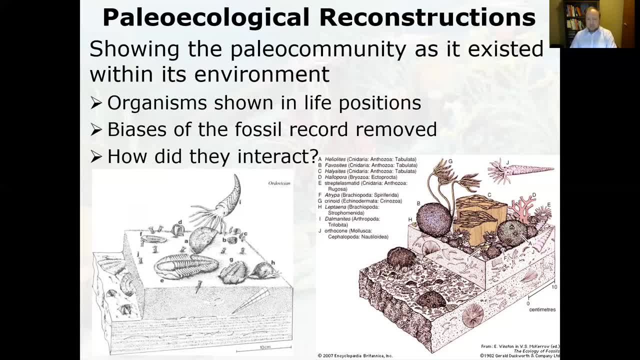 it's all the hard work that's been done to make this work and it's all the hard work that's been done to make this work and it's all the hard work that's been done to make this work. and part organisms. it doesn't look like they did a very good job of kind of backing out the biases. 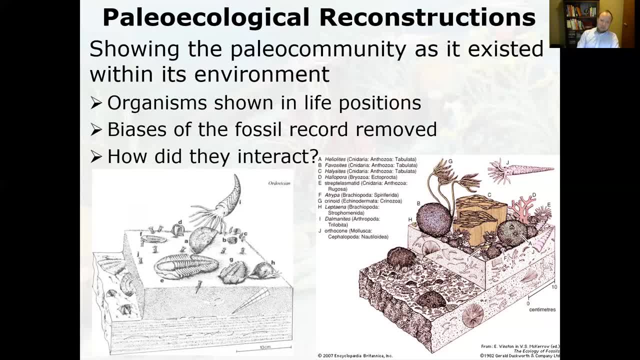 in the fossil record here- and that's always going to be a challenge- there are probably entire species that are just not represented because they wouldn't be preserved. a lot of times, all we see left over are burrows and traces, so remember that as we're reconstructing these paleo communities. 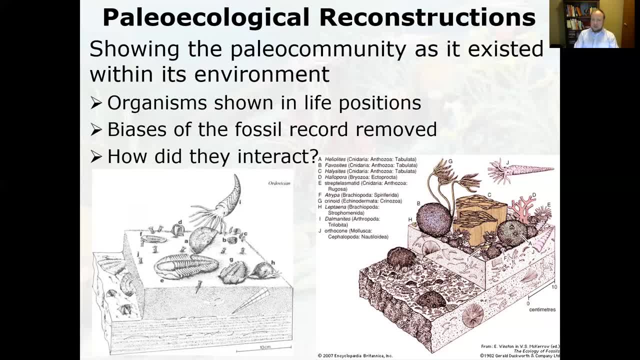 that some of these organisms are just not represented. they're not going to be shown in the fossil record. so we're going to have to do a lot of work to make sure that they're not, and then it's going to make it very hard. there's probably entire tiers of that food pyramid that. 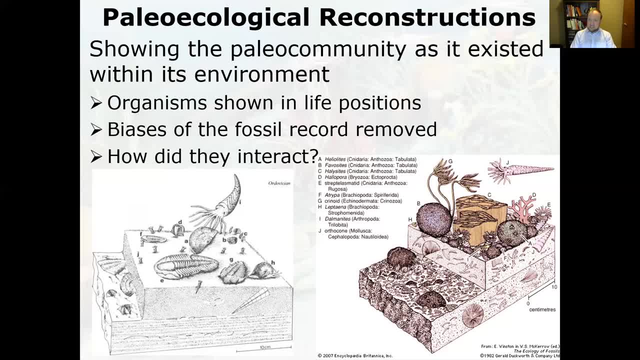 are just not present and we have to kind of look at, well, what do we have to do? we've talked about it before. so you look at modern analogs. we know kind of given ratios of kind of what things should exist in the community. we kind of look at what's filling what niches and that's kind of what we'll. 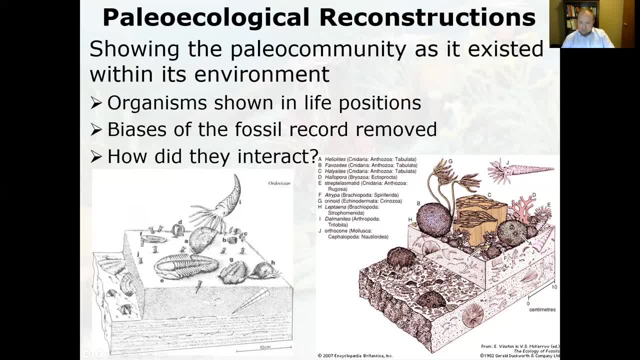 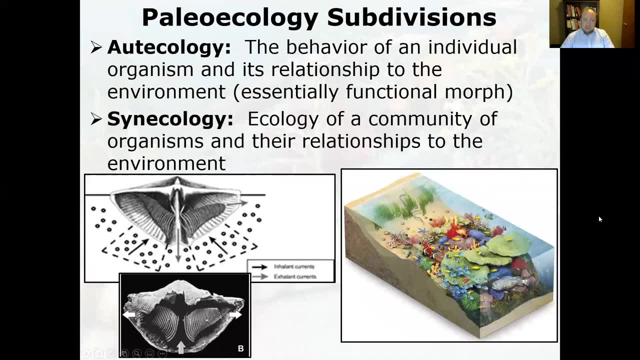 be talking about for the rest of the day today here. but you know, pretty neat, pretty cool to look at a nice little glimpse into the fossil record and then we're going to have to look at what's happening in the past. so there are two main subdivisions within paleoecology, and one is 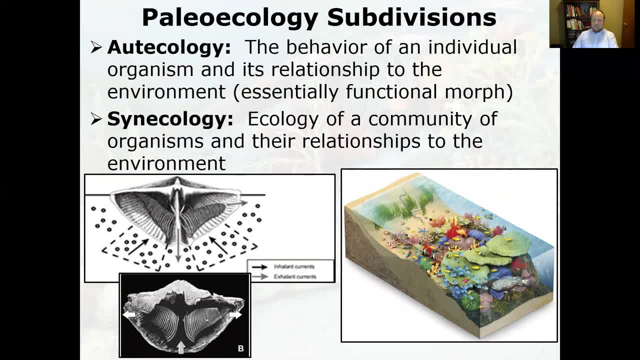 autoecology, which is basically looking at the behavior of an individual organism. it's really shipped to its environment and this probably sounds a little bit familiar to you because it's essentially functional morphology, which we talked about last week. well, two weeks ago now feels like forever ago, but anyway. so here's. 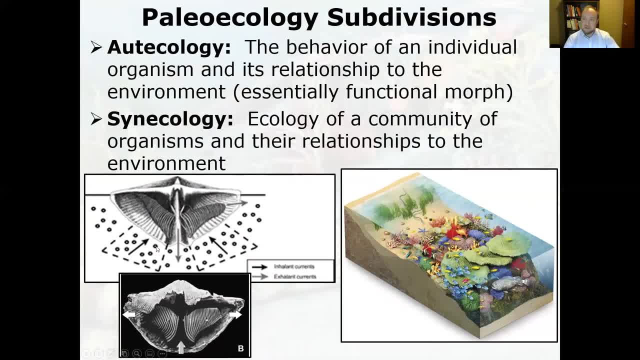 a brachiopod, remember, it's a lofa four eight, lofa four eight. so it has this coiled filtering device, the lofa four, inside its shell. look at these two pictures here. on this one it has inflow from the water column coming in the sides of the shell and then the fold and sulcus of the 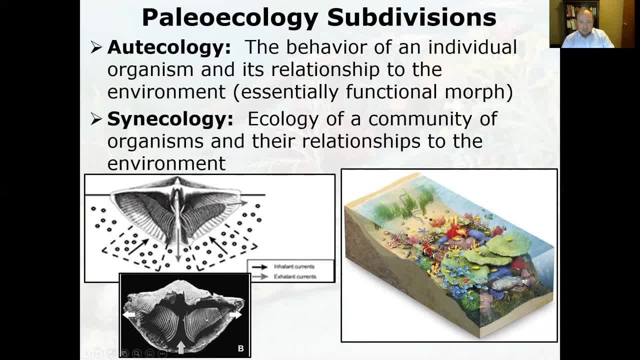 shell that we talked about, kind of using it to funnel wastewater out. so remember these are. these organisms have a u-shaped gut. stuff comes in one end, goes out another end. there is flow differentiation here so that the out doesn't go back in the end. we do not want that on this one, in on the sides. 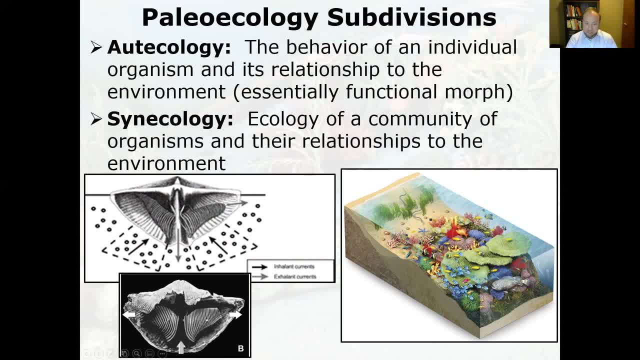 out between the fold and sulcus. on this model here, flow in is through the fold and sulcus and then out through the lofa four, filtered out through there again. this is kind of a problem here, right? so we're trying to study the behavior of these individual organisms and how they 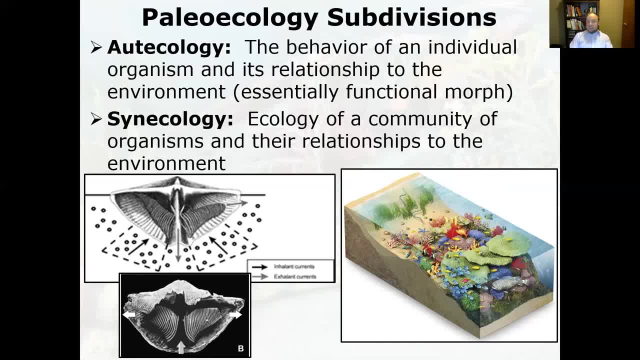 interact with their environment. in a lot of cases it's uncertain. we have the final fossil, we have the hard part- shell. in rare cases we have the internal pieces like this is a very ridiculously good preservation here with some of the internal pieces- like this is a very ridiculously good. 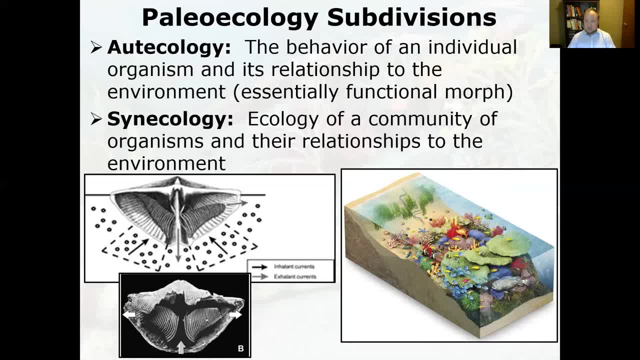 preservation here, with some of the internal pieces like this, is a very ridiculously good preservation. how did this stuff actually work? well, remember we talked about functional morphology. you can just construct a model. try to see how it works. we can look at modern analogs, see how it works, but at the 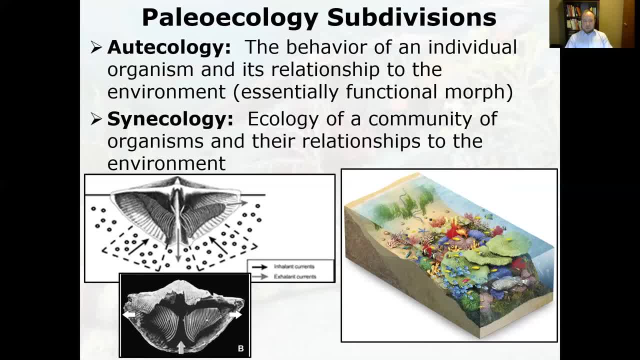 end of the day, maybe we don't know. there's still a little bit of debate about which of these models is right, so interesting. the next one is sin ecology, which is the ecology of a community of organisms and their relationships to the environment. so this is sort of a modern coral. 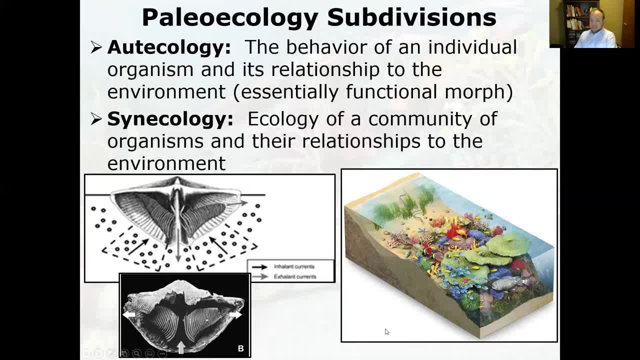 reef environment, and we know just how diverse these coral reef environments are and how complicated the interactions with the organisms are. so like think about like clownfish? uh, clownfish shelter themselves in the anemones, anemones, anemones, anemones. that's the one. yeah, we got it. 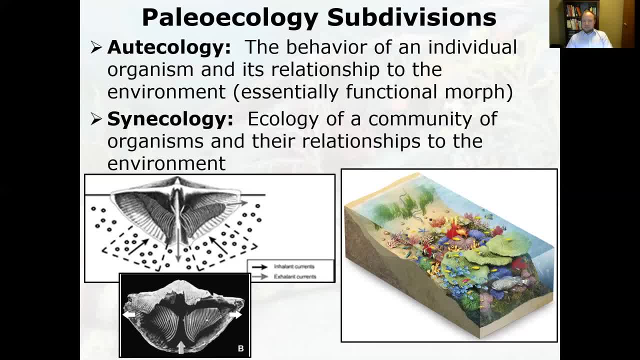 uh, clownfish shelter themselves in there and there's kind of that symbiotic relationship. uh, that sort of complicated relationship is probably lost when you go in paleoecology. we don't get that level of understanding of how these things interacted with each other. um, stuff like zooxanthellae living in the soft tissues of corals and that. 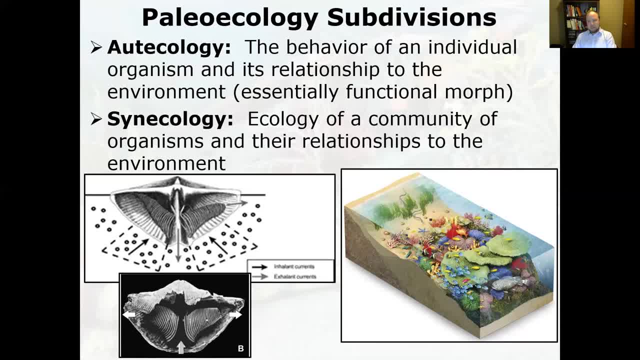 that symbiosis again. uh, soft tissues not preserved, not preserved. things inside soft tissues certainly not preserved, that relationship not preserved. we wouldn't be able to analyze that in paleoecology. so a lot of things are complicating our study here. we're probably not seeing a complete picture. 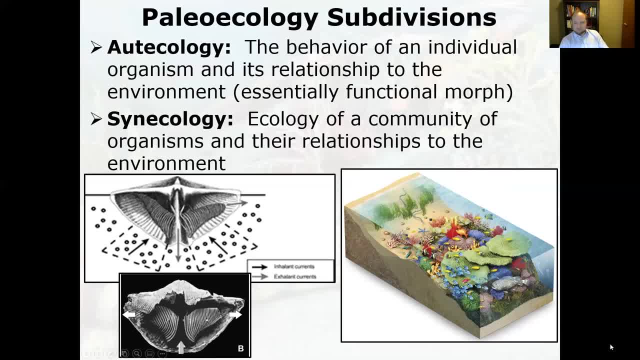 makes it incredibly difficult to reconstruct, and i think it just speaks to the complexity of of these communities and the complex ways that they interact with their environment. even in modern situations where we're able to actually go out and observe directly, it is still difficult to determine this complicated web of interweaving. 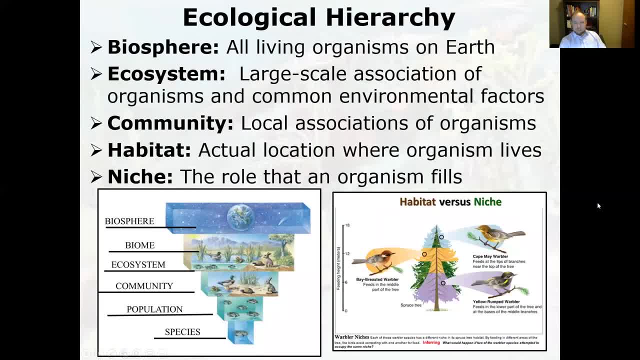 interwoven relationships. so when we're attacking this problem we kind of think about it with this sort of hierarchy. so from the top down up here we have biosphere- all living organisms on earth. talking about ecology at this level is, uh, sort of not very useful. it's just everything, so everything. 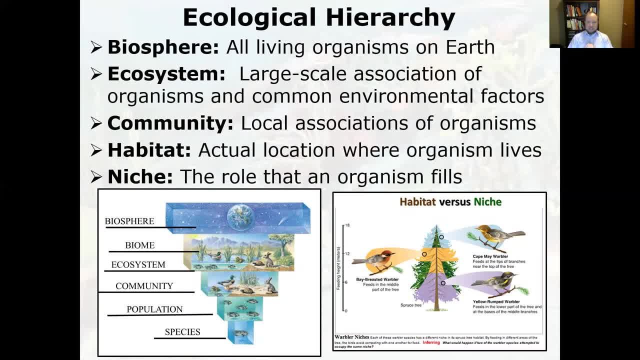 is just everywhere, every living thing, in the sky, in the land, in the ocean, all of the life's creatures down to the next level we have like ecosystems. so ecosystems are like large-scale associations of organisms with common environmental factors. so if you're familiar with the planet earth series, pretty cool, go check it out. so they do like a rainforest episode and like an. 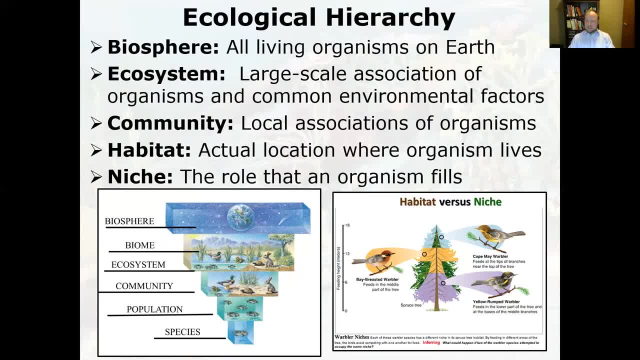 ocean episode, a desert episode, i think, a tundra episode. those are ecosystems. so they're these large, very large scale, kind of global scale bands of very similar environmental factors don't necessarily host the same organisms, but they probably host similar organisms. and then, moving down another level, we've got a community, so local associations of organisms. 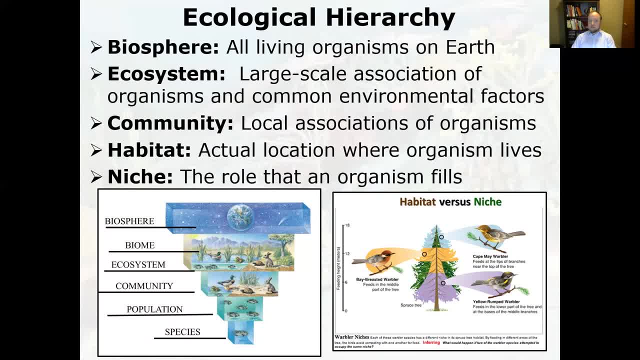 so maybe a forest, or even a particular part of a forest or an ocean or an individual little basin within that ocean. and then, getting a little bit more specific, we've got habitats and niches. so habitats are the actual location where an organism lives. an individual organism lives. 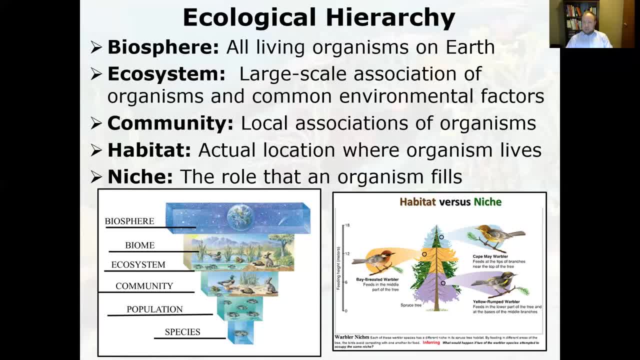 and then a niche is the role that that organism fills, and then a niche is the role that that organism fills. so a lot of people kind of try to frame this as habitat is the organism address, kind of where it lives, where it hangs out, and then a niche is kind of what it does, like its 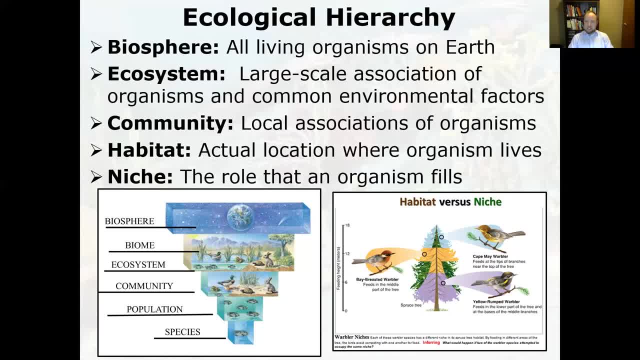 job? what's its occupation? how does this organism actually like, live and interact with its environment on a daily basis? so, for example, here are these birds, which we'll revisit in detail a little bit later: these warblers. their habitat is spruce tree, they live in spruce trees and their niches is basically feeding on insects. 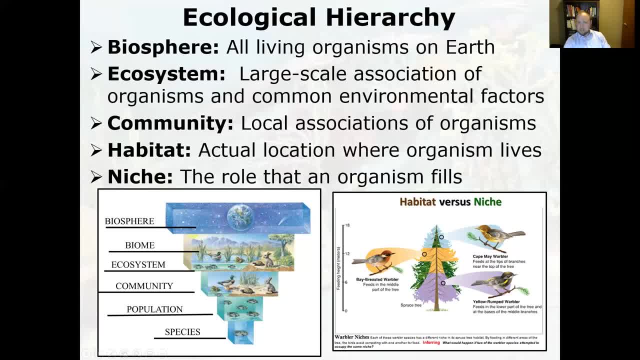 in various parts of these trees. so that's kind of the hierarchy again, working your way up from the big down to the small, and we spent a lot of time talking about species and populations and evolution within those, and now we're starting to move up the ladder, we're starting to talk. 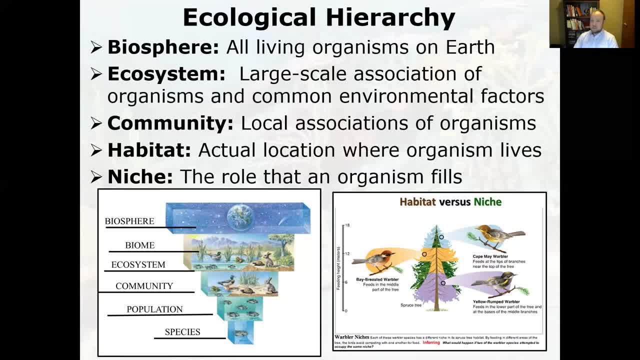 about communities. we're starting to talk about ecosystems. uh, we're probably not going to really talk about the biosphere itself, but i guess we sort of do with. you know diversity curves, things like that. but basically ecology is kind of moving up the ladder to the larger scale things. 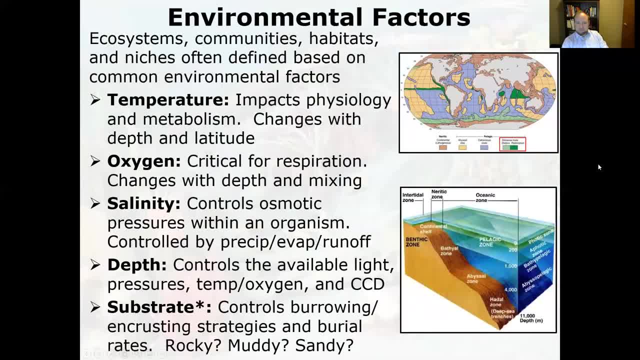 and how organisms are actually interacting with their environment. so what are some things that really matter here? so i said that ecosystems are these like large-scale organisms that are actually interacting with their environment. so what are some things that really matter here? so i said that ecosystems are these like 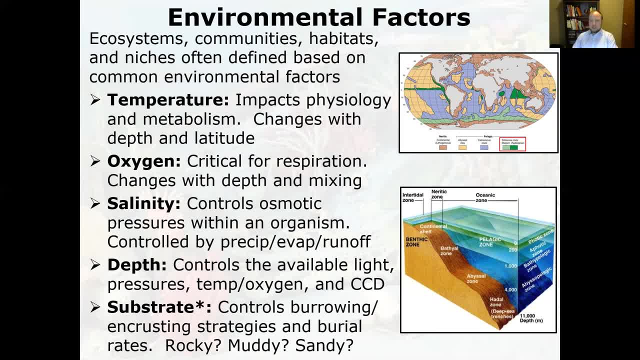 large-scale organisms that are actually interacting with their environment, scale bands of common environmental factors which probably host maybe not the same again, but pretty similar organisms. so we've got a lot of these different factors here. these are the kind of the five big hitters, that sort of. 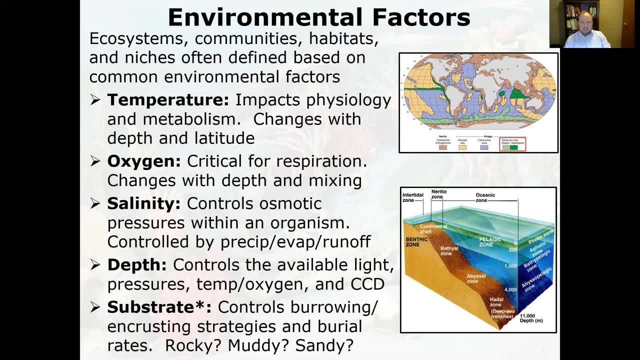 differentiate these, these ecosystems, from each other. so temperature is a big one, so temperature impacts physiology. so we talked about remember how organisms, like sizes and shapes, would change with increasing or decreasing temperature. think back to that lump these video: uh, the big, tall, lanky lumpies in the hot environments they're trying to increase. 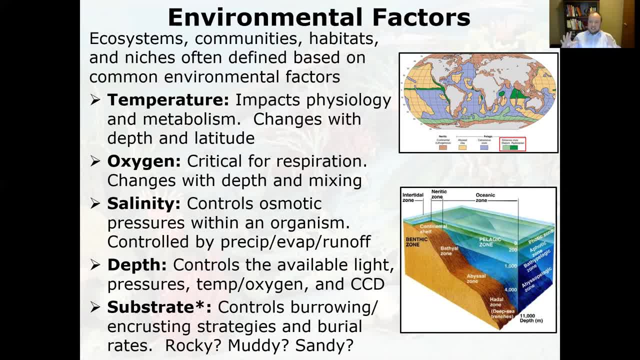 their surface area to get rid of heat, and then the stockier, shorter, lumpy, is a little bit more furry trying to keep in their heat. so temperature matters a lot for physiology, it matters a lot for morphology, it matters a lot for physical traits and it also matters a lot for metabolism. so how, how this? 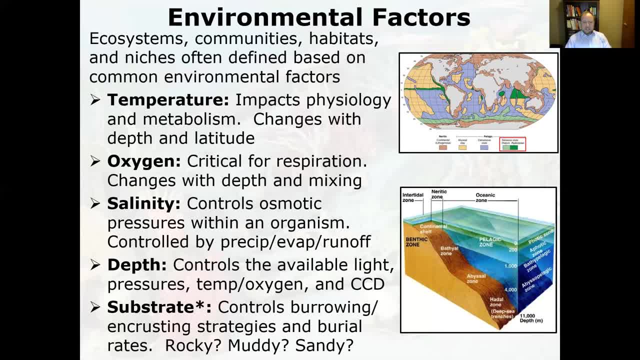 organism is using energy and temperature changes. and again we're going to be mostly talking about the marine environment here because the fossil record, the rock record really again is incredibly biased towards marine. we're stripping things off of the land mostly and putting them into basins. the rock record is biased toward the marine environment so we're using some very high quality. 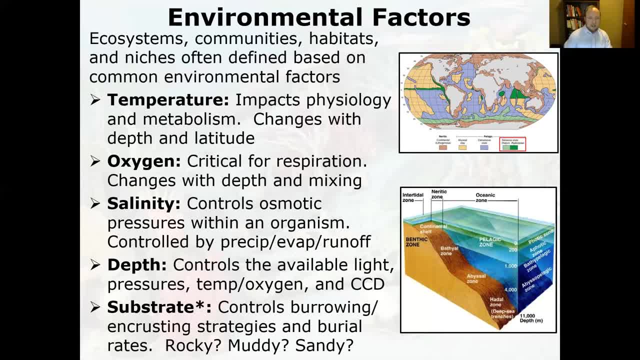 towards being preserved in those basins there. So temperature changes with depth in the water column and it also changes with latitude. So in general, as you get deeper you get colder and in general, as you get closer to the equator you get. 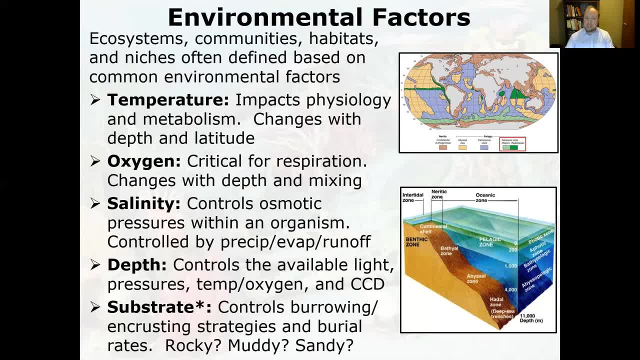 hotter. As you get closer to poles, you get colder And you can see that this temperature has a dramatic impact on paleoenvironment or, sorry, paleoecology. So like, for example, the dark green band, here are radiolarians, So radiolarians. 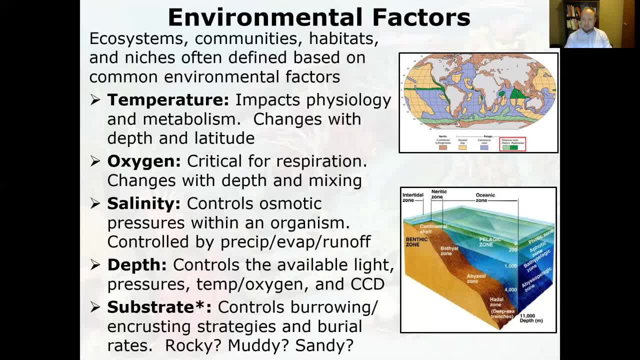 those siliceous plankton that we talked about. they prefer warm And diatoms. the siliceous phytoplankton: they prefer colder environments, And so we get this kind of these kind of like bands. Oxygen is also important, very important. 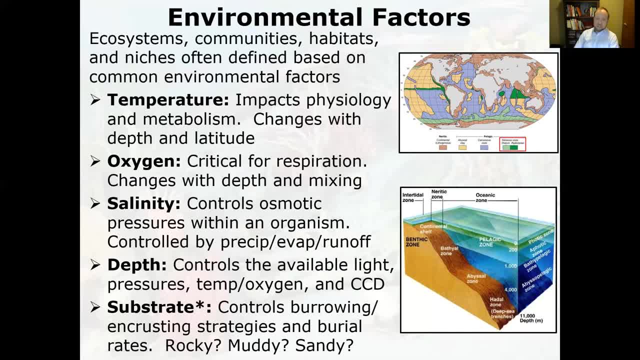 Oxygen is critical for respiration. Oxygen is critical for respiration. Oxygen is critical for respiration. It also changes with depth, but it also changes with mixing. So in areas generally you know, the atmosphere has a lot of oxygen. The water doesn't. 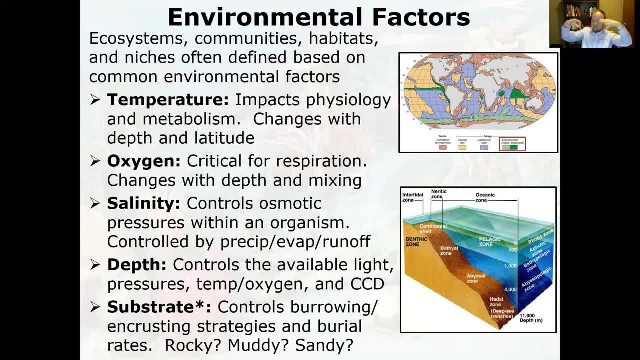 necessarily have a lot Kind of. at that interface. there is exchange, and the more the water is mixed, the more the oxygen is moved around. The more that the water is stagnant. the less that oxygen moves around, the less those nutrients move around, And so mixing can be a very important factor as well. So like 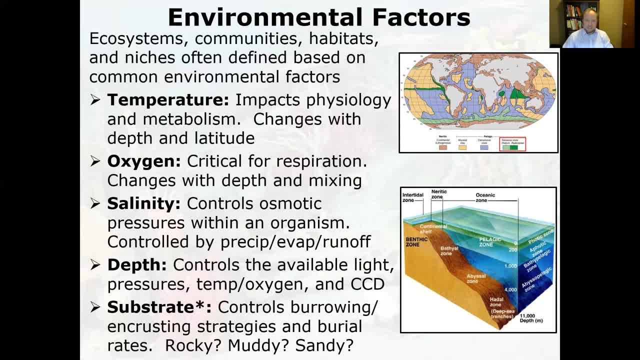 in areas of upwelling, you're able to get a lot more of that stuff in the water column. Salinity is another one. It controls osmotic pressures within an organism. So if you're a saltwater organism, the interior of your body is. 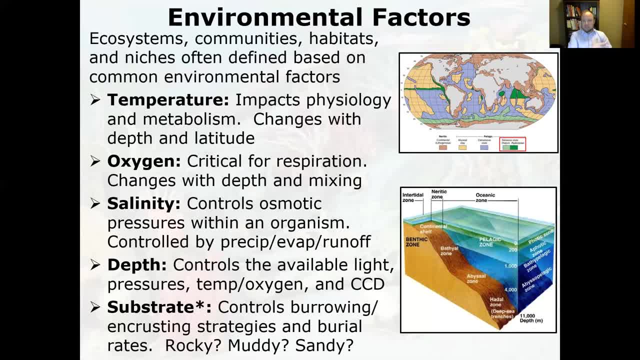 probably less salty than the environment, And so if you're a freshwater, the interior body is probably actually more salty, and so that differential there drives osmosis across their membranes, and it's controlled by precipitation where there's, in areas where there's more precipitation surface sea. 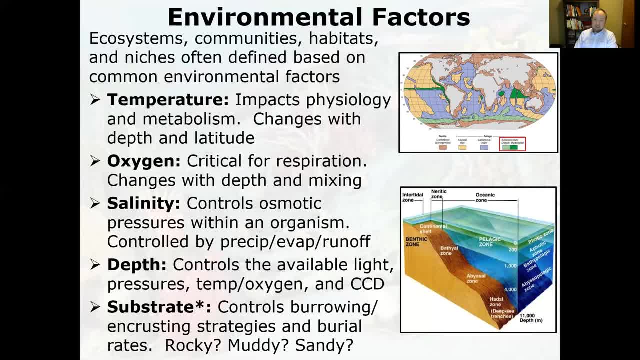 salinities are a little bit lower in areas where there's a lot of evaporation, for example in the like, the horse latitudes, the desert belts of the earth, where there's more evaporation than precipitation, the salinities are a little bit higher. and then where there's a lot of runoff, so like at mouths of. 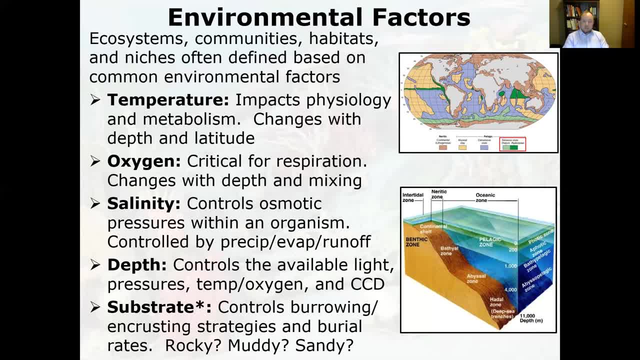 rivers. at glacial outputs, where you're putting a lot of fresh water in, the salinities are a little bit lower. so those kind of things impact salinity and of course, mixing also determines that as well. depth is also a key factor. the depth is a big one for differentiating ecosystems in the marine environment. 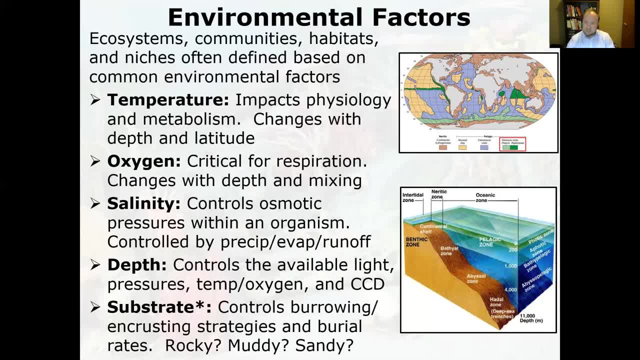 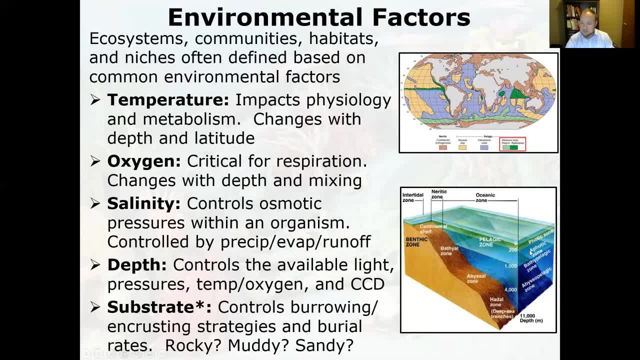 say, like the upper, like 100 to 200 meters. that's the photic Zone, lots of lights able to penetrate. that's where there was phytoplankton, the, the plant plankton and the autotroph plankton. they're making energy in the vibrant. 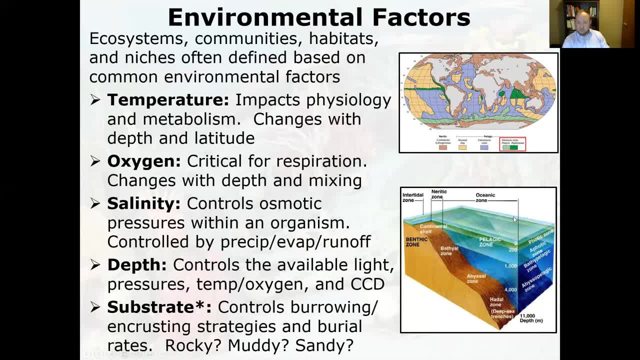 sunlight. as you go downwards through the water column, less and less stuff, less and less lights able to penetrate and eventually you get down into the aphotic zone and this is that cool area where you know, like anglerfish with that cool lantern on their heads, all the bioluminescence, all those neat little critters. 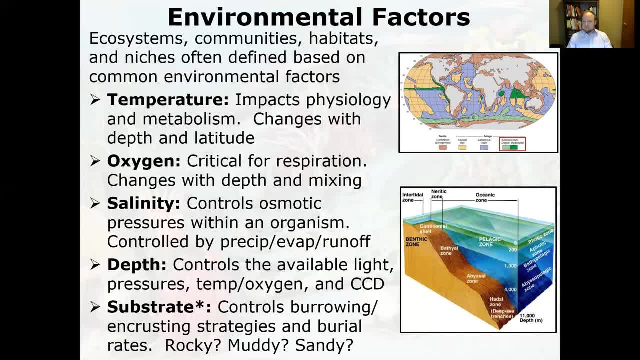 like that. There's no light down there. So how does that affect organisms? How does that affect how they live? How does that affect what they do? Pressure also increases. So pressure increases quite a lot. So think about the Marianas Trench. Only, really, James Cameron and his cool little. 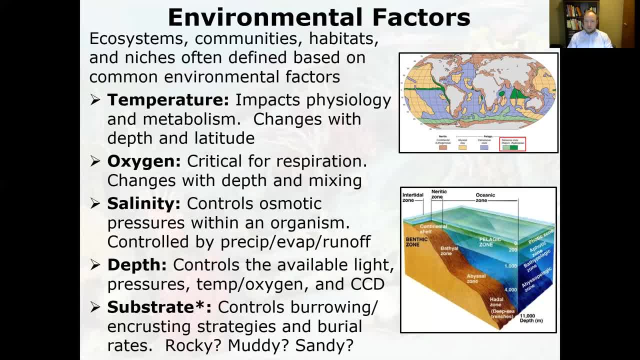 self have been able to get down there, because the immense pressure is down there. Organisms have to deal with that as well. Temperature and oxygen are also controlled by depth, And then the CCD that we talked about a little bit earlier, and we definitely talked about it in sedimentology. 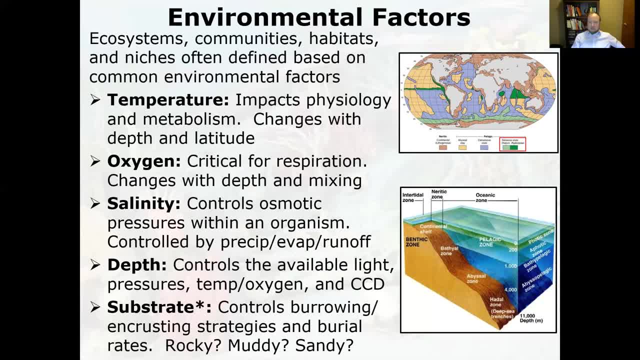 and stratigraphy. the carbonate compensation depth. So that's the area below where calcite dissolves. That's controlled by depth. So remember that marine snow that accumulates on the high temperature, So that's the area below where calcite dissolves. That's controlled by depth. 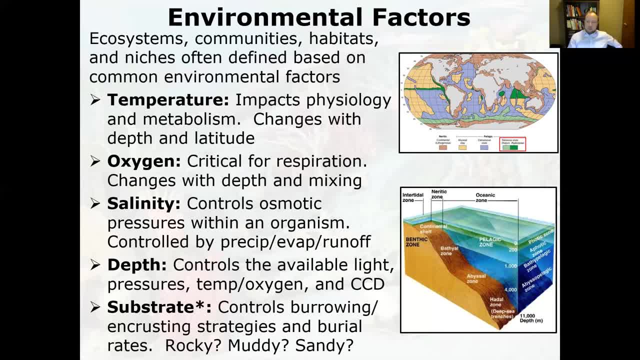 And then substrate what the surface was. So that controls your burrowing strategies. Critters have a much harder time burrowing in a rocky environment than they do in a muddy environment. It controls the kind of burrows that you'll see. It controls the kind of encrusting strategies. So 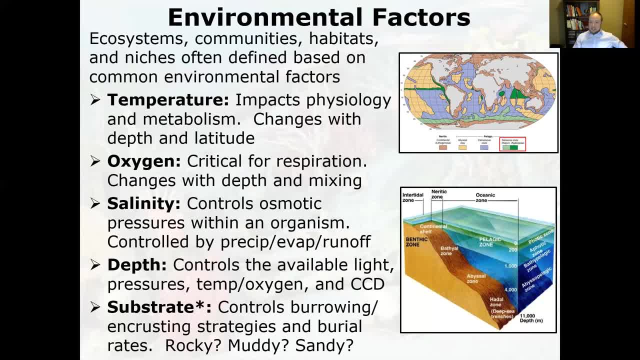 like a lot of organisms need to encrust on hard rocky substrates. If it's a muddy substrate, they're not going to be able to live. It also controls the burial rates. So think about, like a very sandy environment with a lot of clastic input, An organism that doesn't have a mechanism. 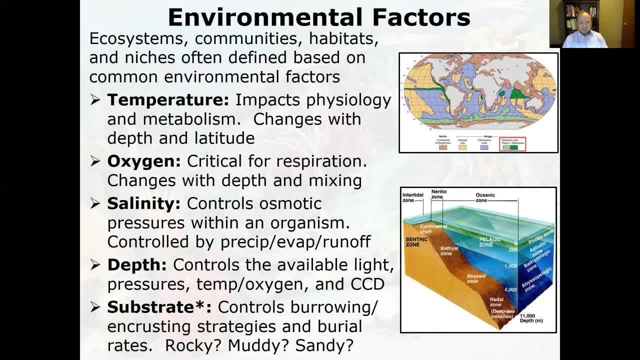 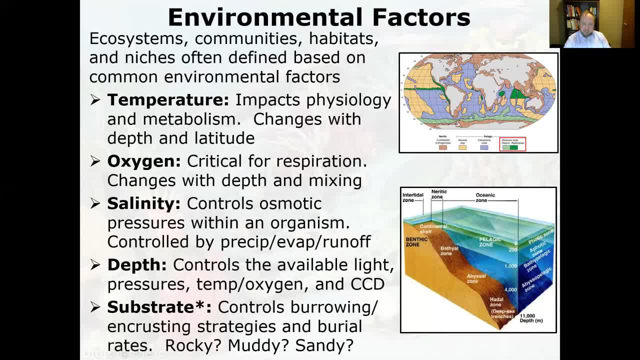 And there's a little asterisk here because, again, thinking back to paleoecology, we are looking at the rock record, We're looking at the fossil record. How do we get to these factors? Well, substrate's the only one that we can directly observe. So we look at the rock. 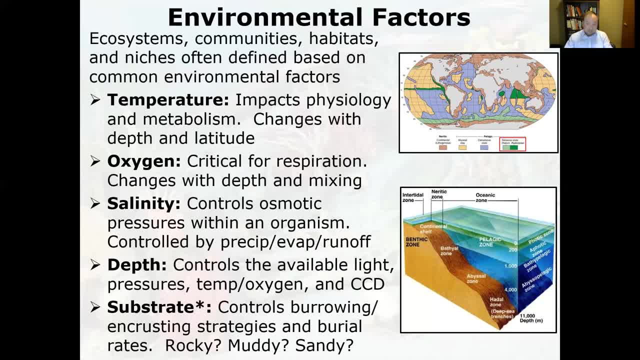 presuming that that's the sediment that they were actually living and engaging with in life. there are instances where organisms are transported out of their environment, so all bets would be off at that point. but presuming that the organisms are preserved essentially in life position, or at least in their life. 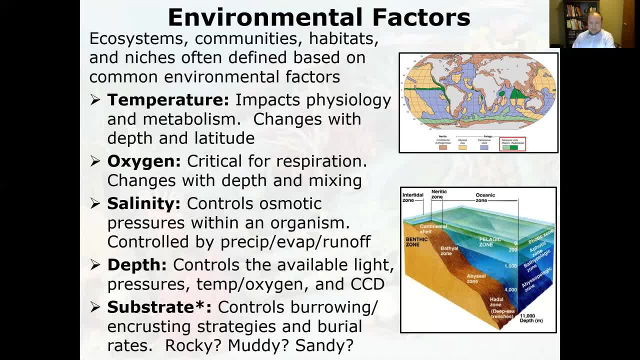 assemblage. that's the one that we can look at. we can see like, oh okay, well, this was a hard, this was a hard ground, or this was a sandy bottom, or this was a muddy bottom. it's the only one of these factors that we can really get to. 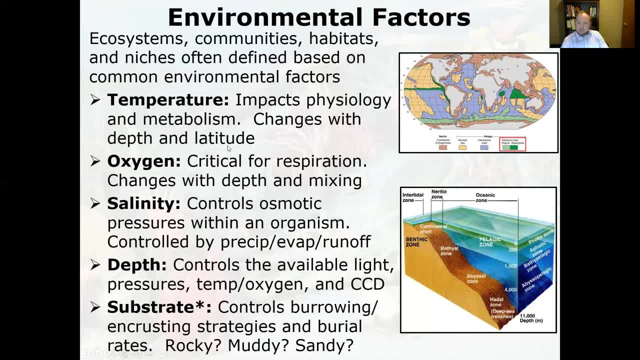 temperature. there's a couple things we can look at again. we can look at the morphology of the creatures because we kind of know some patterns to get like a proxy for temperature, oxygen in some cases. we can look at isotopes, salinity. again we can kind of look at chemistry but depth, so that's very important. we 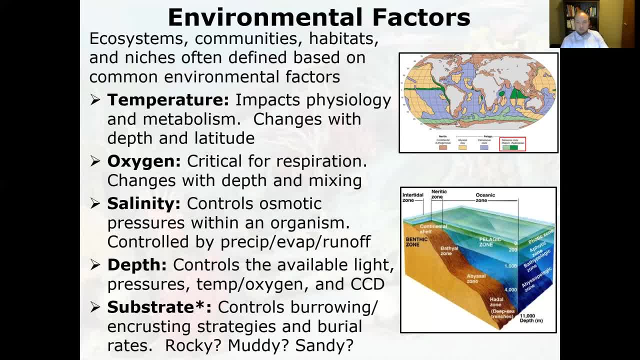 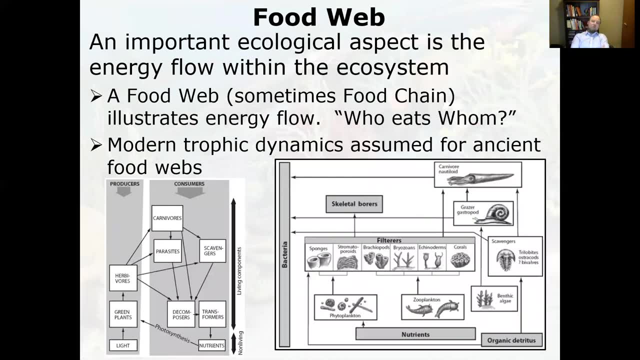 can look at sedimentary structures to try to identify inferred depth, but pretty difficult. so when you're studying paleoecology, these five factors pretty tricky. so another concept here is food web. we've talked about this a little bit before. food web is a very important aspect. it basically 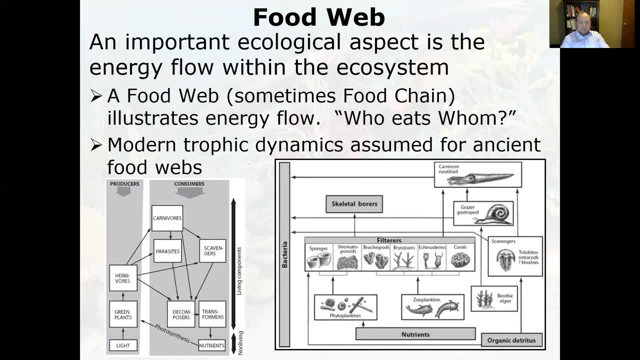 shows the energy flow within an ecosystem. sometimes you'll hear this referred to as the food chain. food chain is a little bit oversimplified. it sort of implies this like linear up, and we know that it's a lot more complicated than that. but basically this food web is is essentially who's eating. 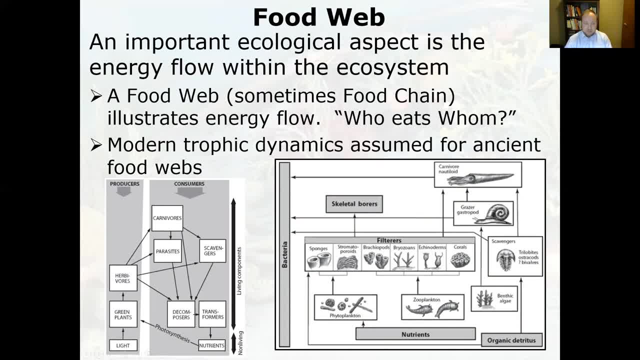 who where's the energy moving through the system? so at the bottom here we have non-living things, nutrients. we also have non-living thing, light. you take some nutrients, you take some light, you get some photosynthesis and you get these green plants in the marine ecosystems. those green plants are the phytoplankton, so your 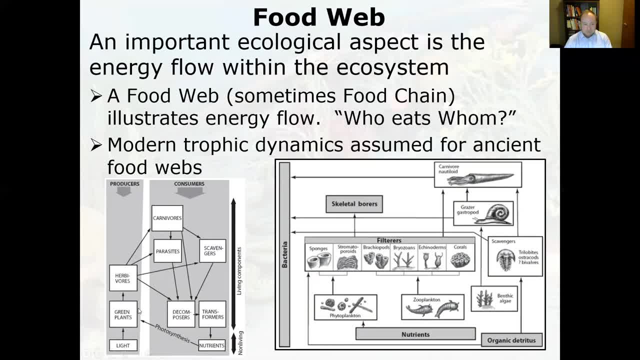 diatoms, things like that. the next level up are the herbivores, the things that eat those, and then you've got all these other various components going on here. so there's been a lot of attempts to sort of like: look at ancient environments and try to reconstruct their food web and again remember how many assumptions are. 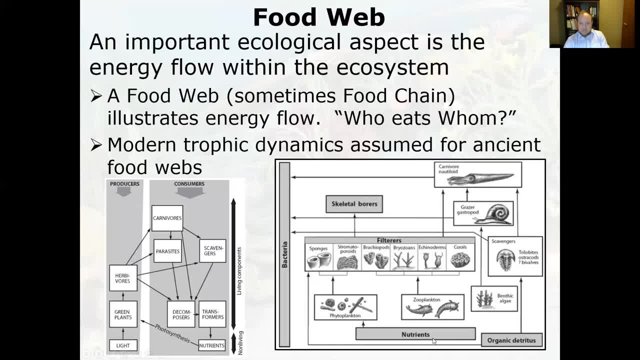 going into this. but we have sort of the same model. we kind of assume that the present is the key to the past. so how do you reconstruct an ancient food web? you look at modern food webs and you sort of try to assign roles to these ancient creatures. so like down here, this is for an ordovician reconstruction- nutrients. 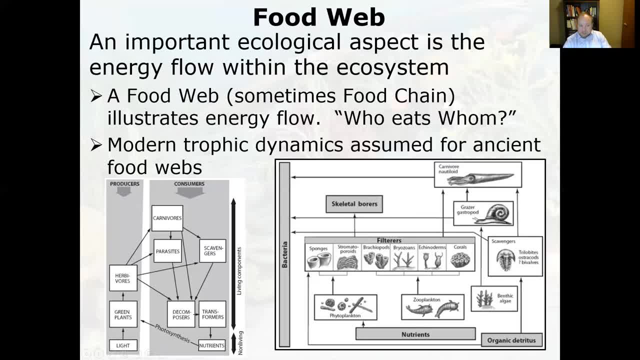 that probably didn't change. the bottom of the food chain are these inorganic nutrients, light things like that phytoplankton, utilizing those zooplankton, feeding on the phytoplankton. the first level up on the chain here are the filter feeders. today, oceans are dominated by corals and bivalves, not really the case in the 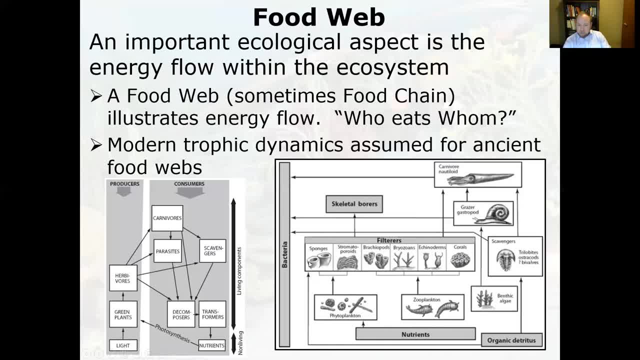 ordovician sponges and stromatoporoids, much more important. brachiopods, a lot more important than they are now. crinoids, they're everywhere and corals are there in general. they're the kind of solitary rugose corals, but they. 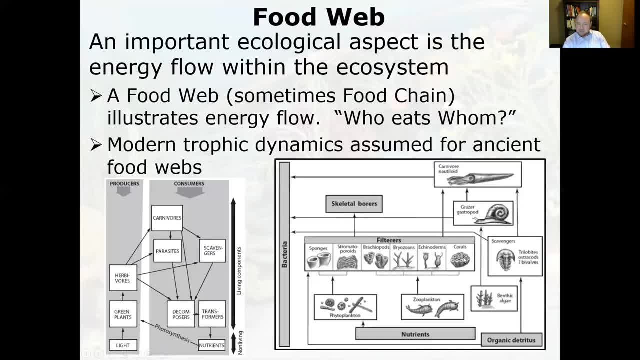 are present, they're just a relatively minor part. so remember, the organisms that fill these niches, fill these roles, changes through time. we've got trial bites kind of scavenging around skittering through the mud filter feeding- or I should say deposit feeding- out of the mud. we've got gastropods kind. 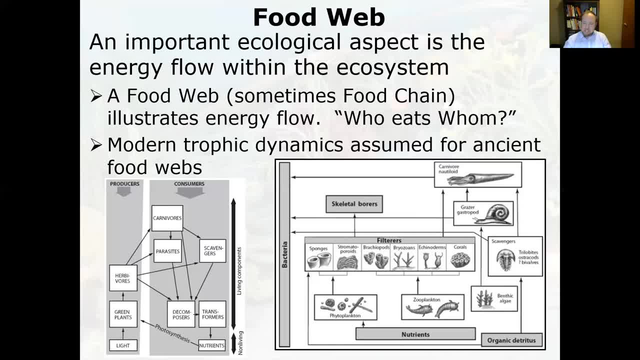 of grazing around, eating algae, maybe even boring in the skeletons, boring in the shells, and then we've got at the top here, the apex predator of the ordovician, the orthocone nautilus. so we've seen some shells of these things, one of the specimens that we looked at. 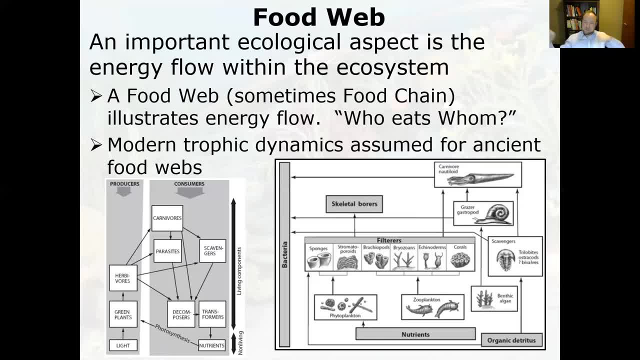 in lab was like that big, but it was only a small part. some of these things can get quite large. they are the apex predators of the ordovician. really not a lot of apex predators, you'll notice. still think about the ordovician and the apocalypse. we've got a lot of apex predators. what's happening today is 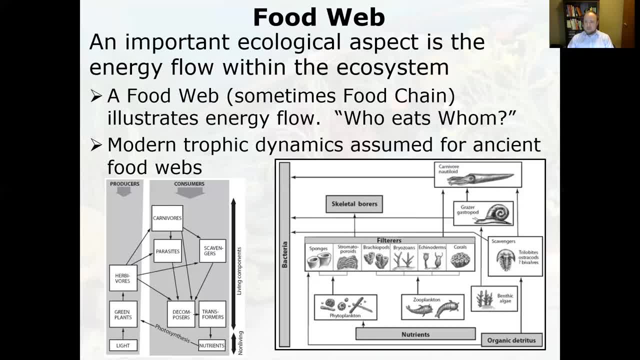 that they're all part of the same species. so when we think about like a modern ocean, think about: we've got orca, sharks, dolphins, we've got all these various wide diversity of high-level predators that didn't really exist back here. so we're gonna talk a little bit next class about some changes that we've. 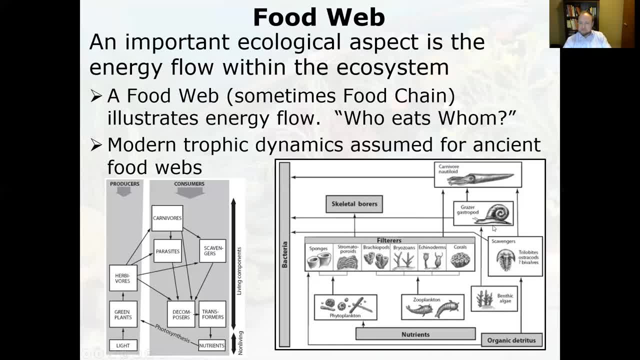 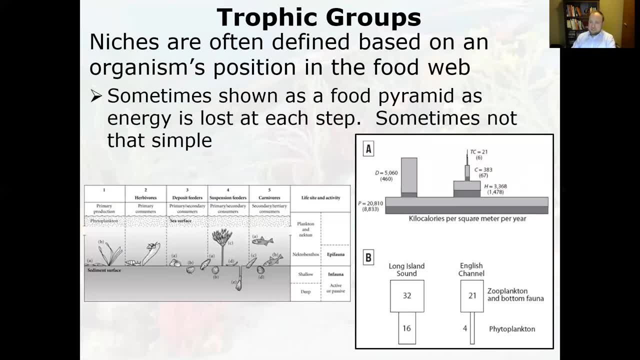 seen through time, with environments and- and that's kind of one of them is like- and just some sort of interesting changes through time. So, talking about these trophic groups- we talked about food web- There's also kind of this concept of the food pyramid. 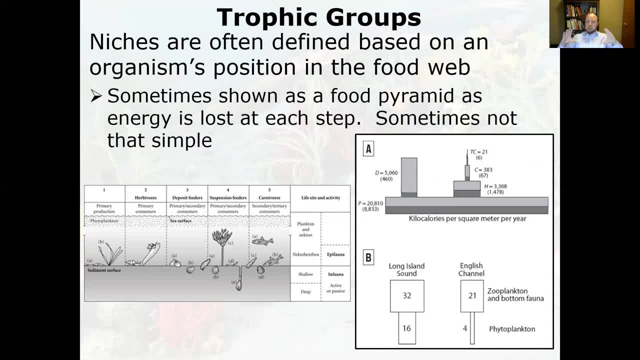 So we've talked about. you know, at the bottom you should have a nice wide base, the primary producers, And then, as you move up towards the apex, predators. energy is lost at every step, And so there's less and less biomass as you move up. 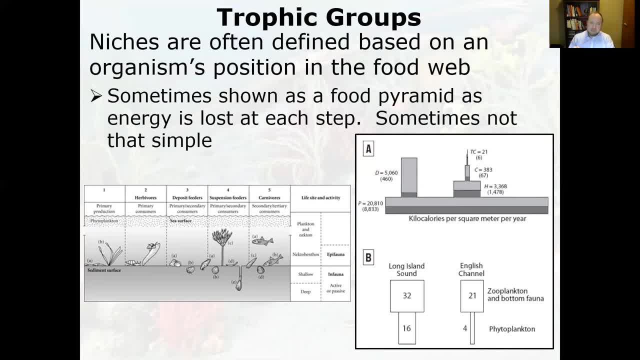 And there's less and less individuals as you move up. That's not always exactly true, So like, for example, this: here is an example that shows: okay, this is a food pyramid that we would sort of expect. We've got this wide base of P as producers. 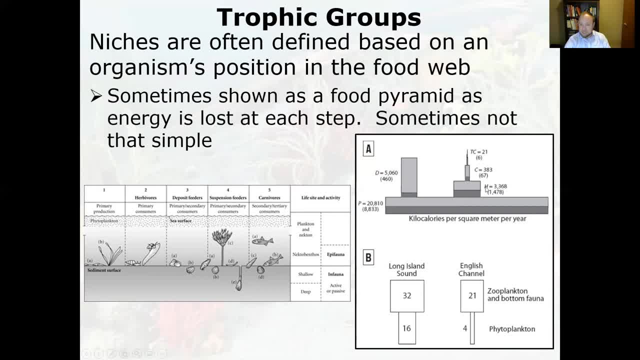 Above that, we've got this slightly less wide base. well, substantially. So we've got this substantially less wide base of herbivores that feed on those producers, C is, the consumers, And then these are the top carnivores, And so you see the wide base tapering to the top. 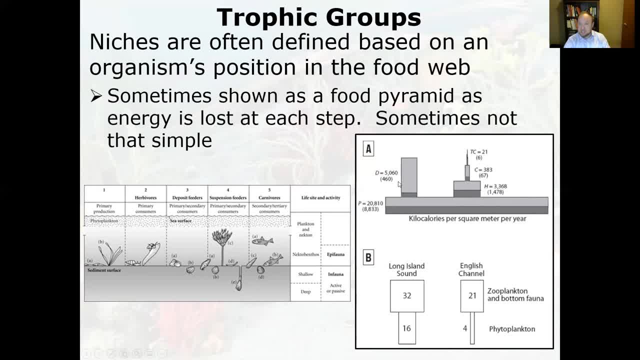 kind of what we'd expect. Decomposers are over here. They're kind of just feeding on everything once it's kind of served its purpose and propped. So this is kind of what we'd expect. But looking at some modern environments, 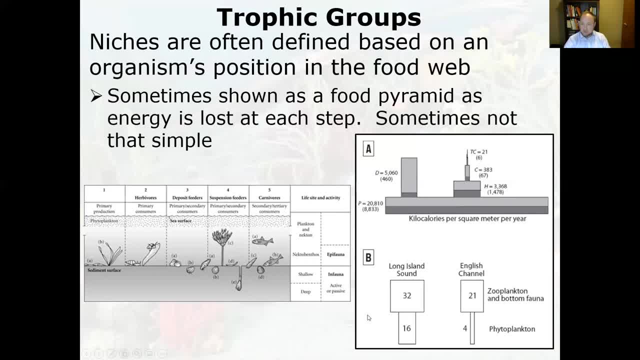 some modern environments, particularly marine environments, we can actually get this kind of like upside down pyramid which, when you think about it initially doesn't really make a lot of sense. So, for example, Long Island Sound biomass of the phytoplankton is about half that. 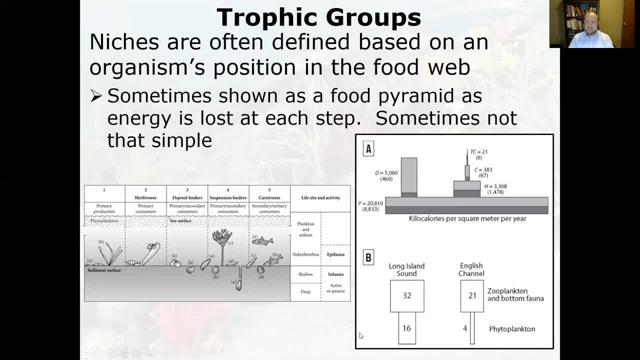 of the biomass of the zooplankton. So the zooplankton and the bottom fauna, the benthic filter feeders, they're feeding on this phytoplankton, but there's about half of that with respect to their biomass. 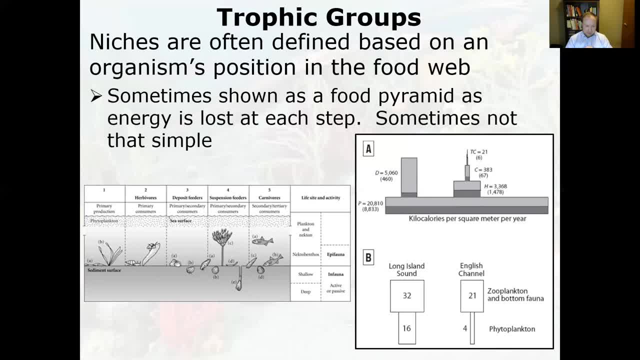 So how does that work? Well, think about like growth rates. So think about how long an apex predator lives, Think about how long an herbivore lives versus how long an individual phytoplankton might live. So these phytoplankton are relatively low in numbers. 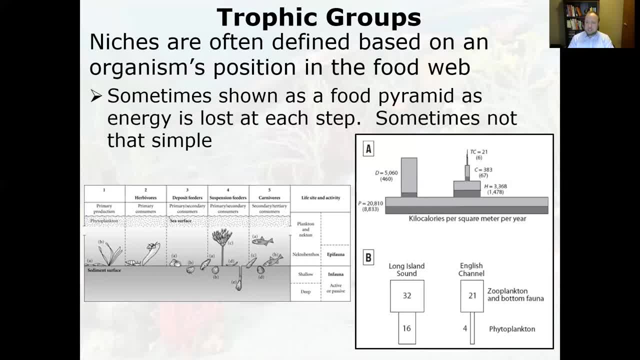 but as they're cold, they're replaced very rapidly, And so this allows us to have this sort of like upside down pyramid, and the whole thing doesn't topple over, because- think about Jenga- you remove a block, imagine, you just put it right back. 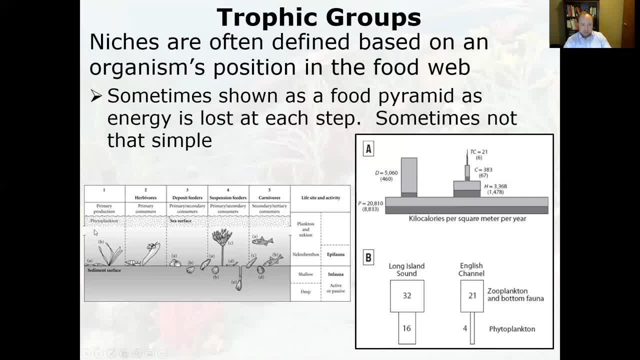 And this is kind of a schematic here: primary production: phytoplankton in the water column, shallow in the water column generally, or also maybe some growing right on the sea surface and relatively shallow waters or, sorry, sediment surface. So we've got herbivores feeding on that deposit feeders. 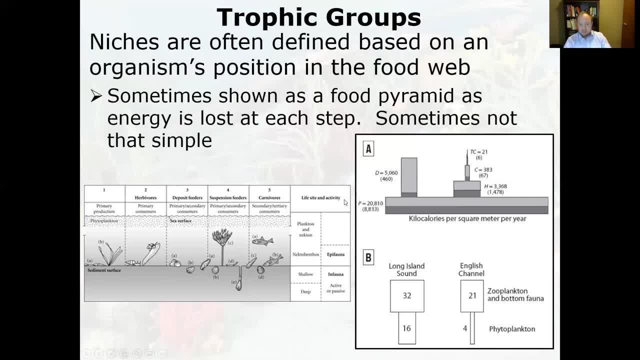 and then we've got the suspension feeders, carnivores, And then we also see kind of these life-slighten activities. So there's in fauna things that live in the sediment, shallow and deep in fauna. These guys are slightly low in the sediment. 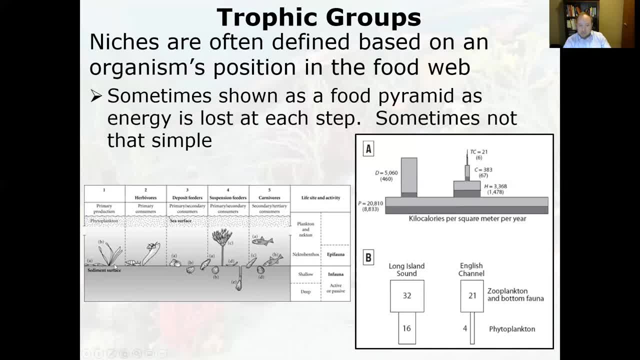 These are deeper. There's epi fauna, things that are right on the sediment, And then there's the plankton and the nekthos that are swimming or floating in the water column. So there's kind of this like 3D aspect to the environment. 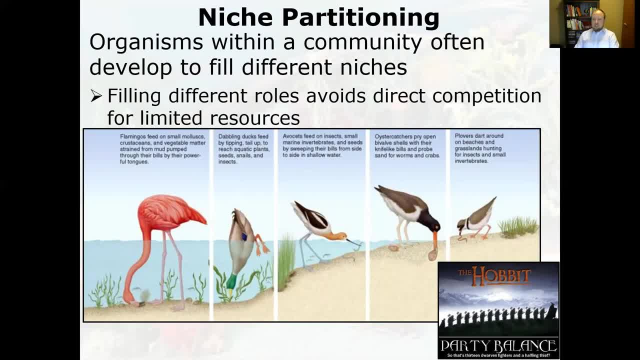 So why do we have niches? Why are there different roles within a community? So the whole reason here is that if there's a lot of different organisms, they're competing for limited resources. There's only so much food present in this particular ecosystem. 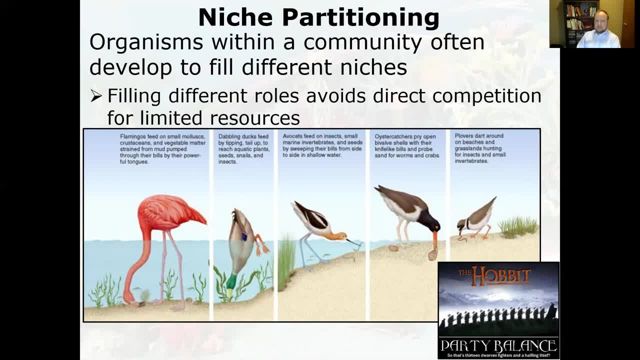 So if everyone's trying to get their fair share, it's best if they avoid direct competition with each other for these limited resources. So think about toilet paper. right now, Toilet paper is a limited resource. If we were somehow to avoid competition to it. 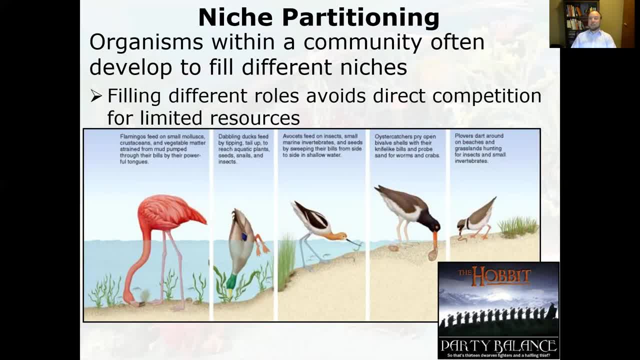 like say, a lot of people in a lot of other countries have bidets. they're not necessarily fighting for the toilet paper resources. So this is a really neat example here. So this is a really neat example here. So this is a really neat example here. 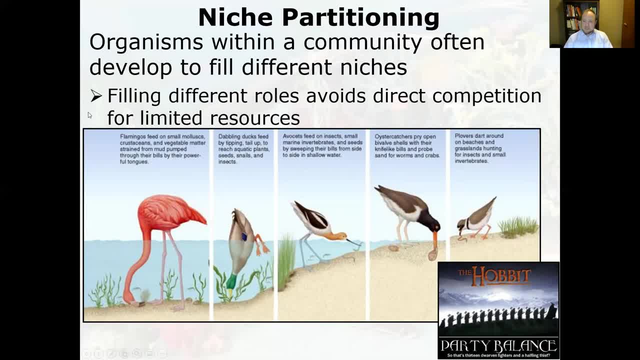 Of some different birds that coexist within the same community And superficially, OK, they're birds and they're digging stuff out of the dirt or eating plants right in the dirt, And we would kind of think, well, OK, well. 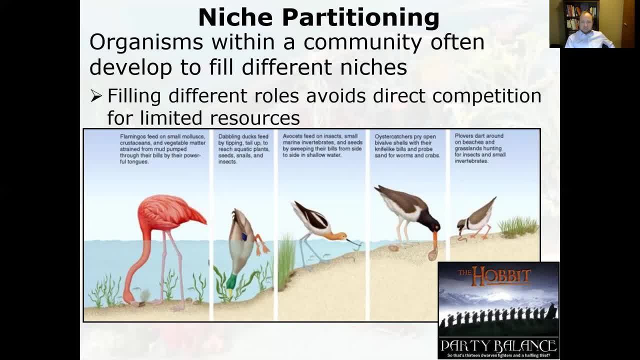 they're fighting for the same resources. But if you look at it a little bit closer- and again, this is very easy to do with a modern environment where we can go directly observe- a lot harder to do with an ancient environment- we can see that 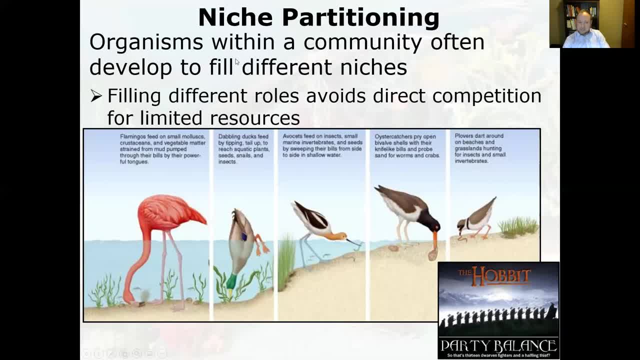 They're actually behaving quite differently or doing things quite differently. So, like the flamingos with their long legs and long neck, they kind of dig into the sediment, kind of shake their heads around and filter stuff out with their filter feeding beaks. They're exploiting things in the slightly deeper water. 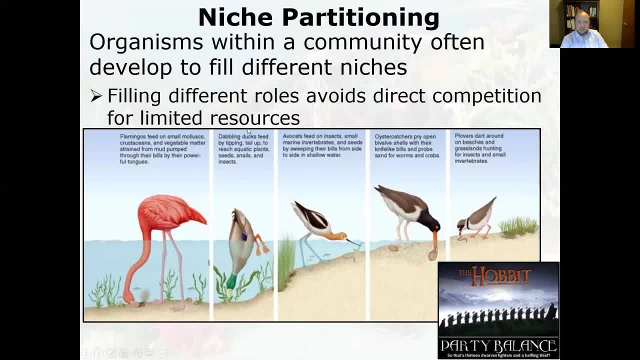 and exploiting things kind of in the mud. The ducks dive down. They're exploiting things that are kind of on top, In most cases just on the top, The epi fauna, These avocets. they're feeding on things kind of in the shallower water. 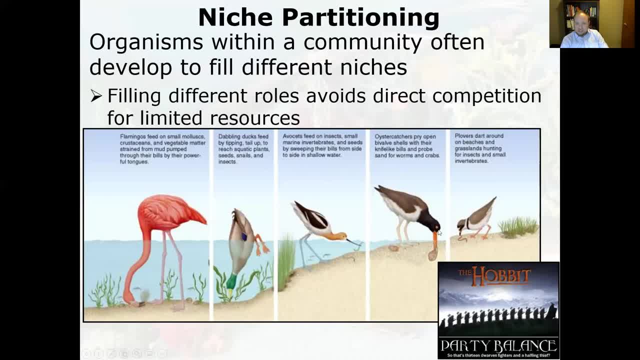 They're not able to reach deeper. like the flamingos, Oyster catchers tend to be in the really shallow water And they're going after the bivalves in the sediment And then the plovers are kind of chasing around stuff that's on the sediment. 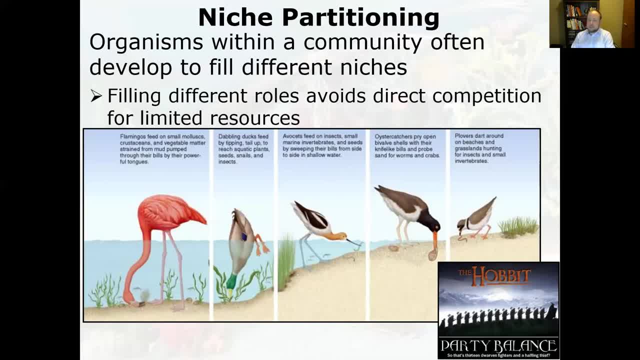 So superficially it looks like, hey, these critters are all fighting for the same resources, but they're really not. They're all filling different roles and, at the risk of letting my nerd flag fly, think about an RPG. So an RPG, a party- is much more effective when it's balanced. 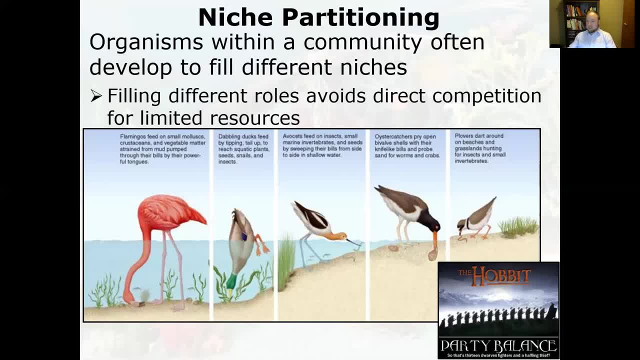 So say a tank and maybe some ranged throwers, wizards, something like that. So the joke here, like the Hobbit. So the party balance: There's 13 dwarven fighters, a halfling thief and a wizard, whenever he feels like it. 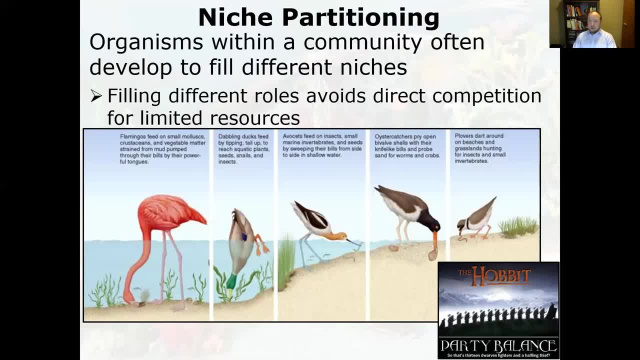 So there's 13 fighters fighting for The same role. fighting for the same item drops. fighting for the same kills Communities. try to avoid that by filling different niches, trying to find kind of balance. There is only so much resource to go around. 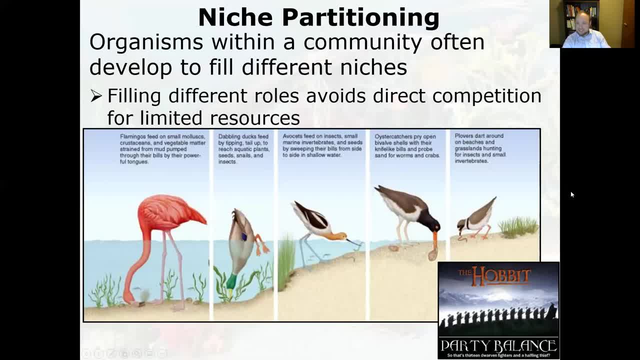 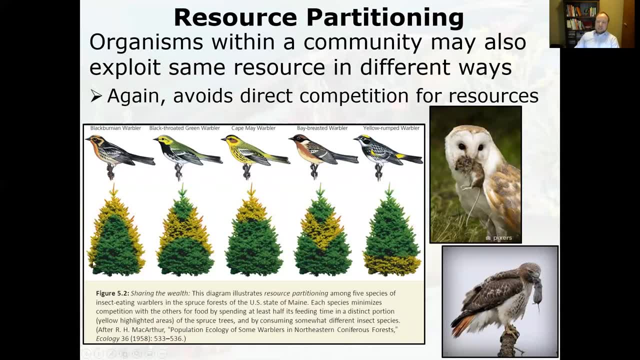 Everyone wins when you're able to kind of share. I suppose is a good way of looking at it. Another thing that we're able to do is resource partitioning, So organisms within a community, they might also exploit the same resource, that same limited resources. 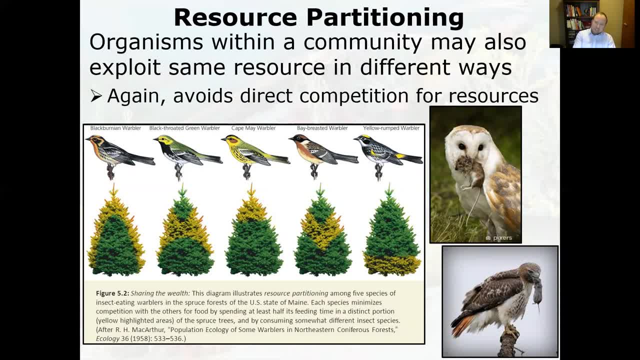 But they might do it in different ways. So niche partitioning things, we're exploiting slightly different resources. Resource partitioning is exploiting the same resource but in a different way. So one cool example of this are these warblers. And again, looking at these warblers, look at their beaks. 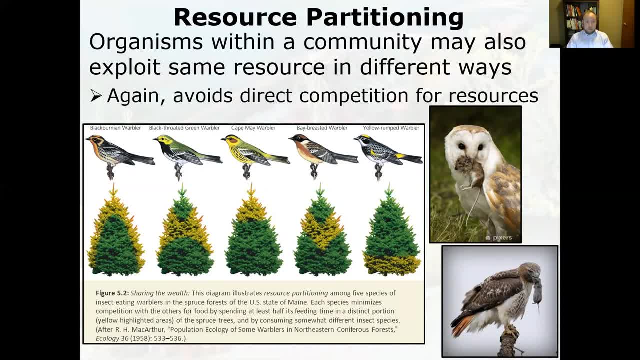 Their beaks are very similar. Look at their morphology There. Their morphology is very similar. The only real difference is their coloring. I'm actually not sure if that's significant or not. I'm not an ornithologist, But interesting nonetheless. 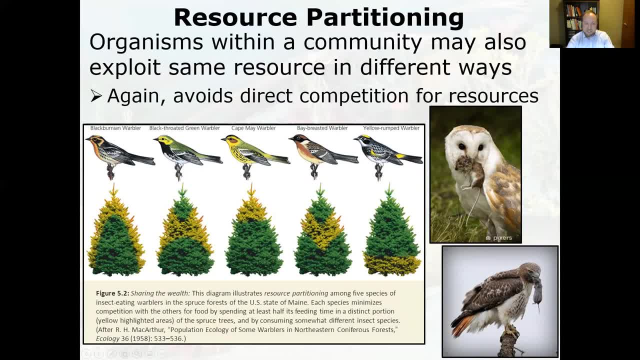 Not preserved in the fossil record though, But pretty interesting. Looking at these birds, they're superficially very similar, They do very similar things. They eat insects in spruce trees, But to partition that resource, so they're avoiding competition with each other. 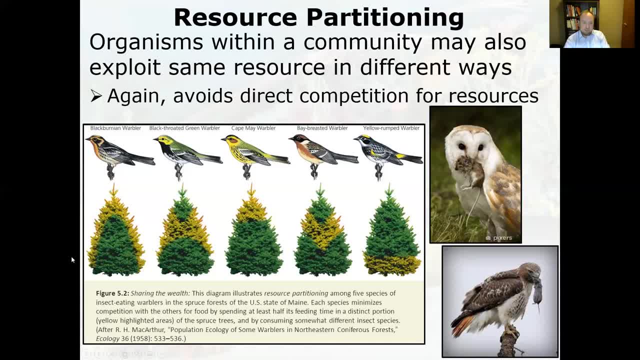 avoiding fighting over those individual resources. they exploit in general different parts of the spruce tree, And so they come into a lot less direct competition with each other, a lot less swabbling. So think about countries. Borders are a somewhat artificial concept. 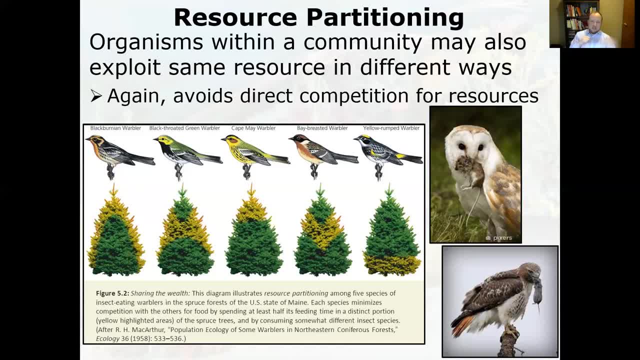 But it kind of helps us from swabbling over resources. Obviously, we still fight over borders And we still fight over resources, But probably a little bit less so when we know that, well, this over here is this country, This over here is this country. 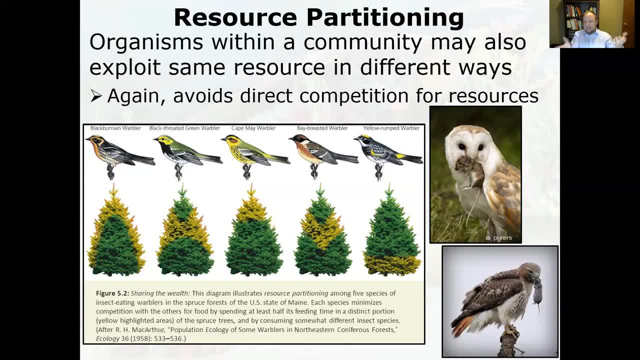 These are my resources, These are your resources. It kind of helps to sort of lessen that fighting, that swabbling that back and forth, Makes life a little bit easier for everyone, unless of course you're on the other side of the resource. 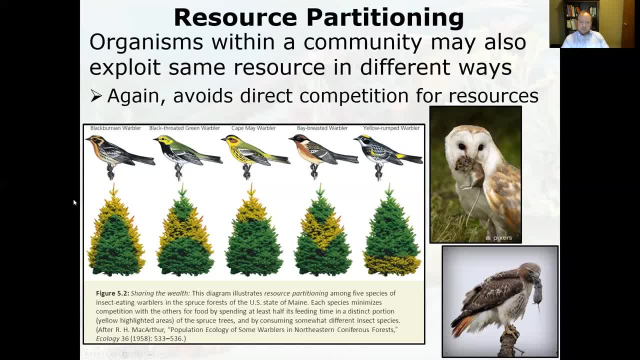 equation. So these are sort of exploiting resources in different places. There is also this concept of exploiting resources at different times. So think about a hawk. This hawk has caught a disease. It's a delicious mouse. Nom, nom, nom, nom, nom. 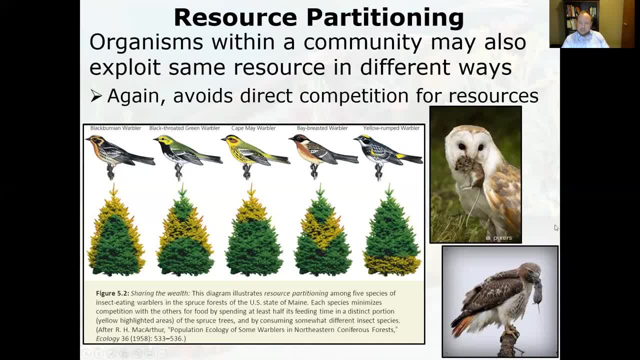 This owl has also caught a mouse. The hawks are hunting during the day, The owls are hunting at night. They're fighting for the same resources, But they're not fighting for it at the same time, So they're not really in direct competition with each other. 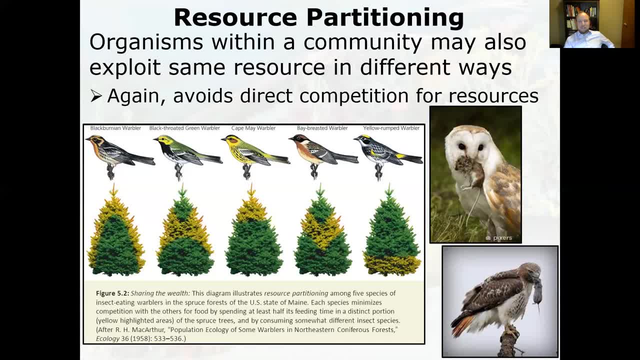 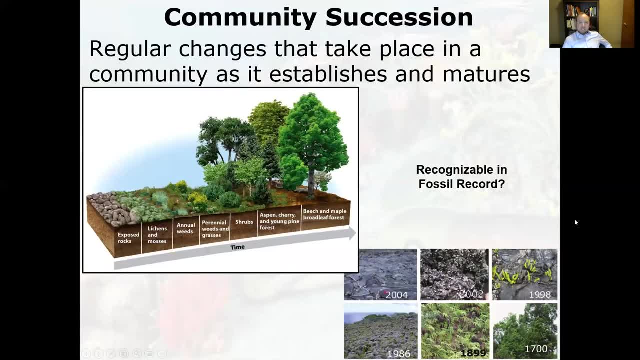 Bad day to be a mouse looks like there, And I don't know if it's ever a good day to be a mouse, But let's see. Another common concept in ecology is this idea of community succession. So community succession, are these regular changes? 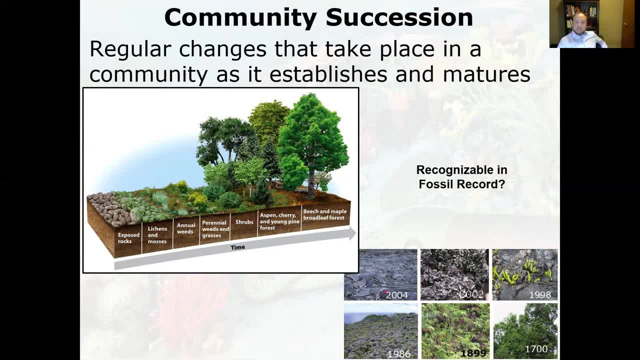 that take place in a community as it matures, as it establishes itself and matures. So think about going from bare exposed rock so like a lava flow or a landslide or something completely strips, or a fire completely strips the vegetation. 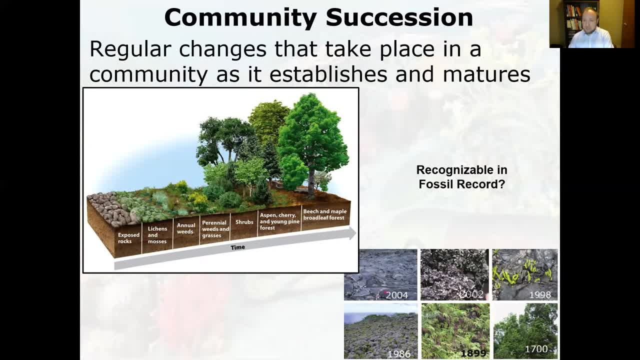 And then the community rebounds, But it doesn't do so right away, It does so in stages, right. So we start with exposed rock And then the first thing to move in, the pioneer species are like lichens and mosses and ferns. 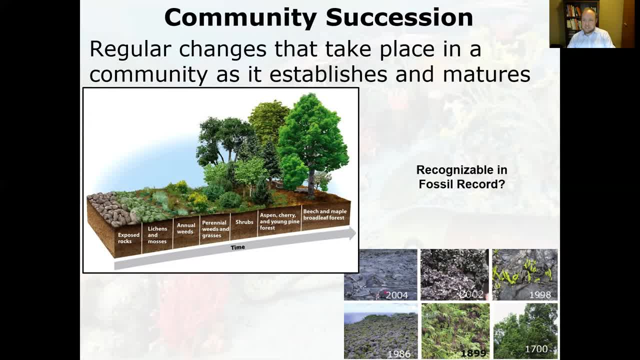 So remember we talked about mass extinctions. One of the first things that we see moving in after a mass extinction are ferns. The large plants are dramatically reduced And we're sort of starting over from scratch And we see the lichens and mosses and ferns. 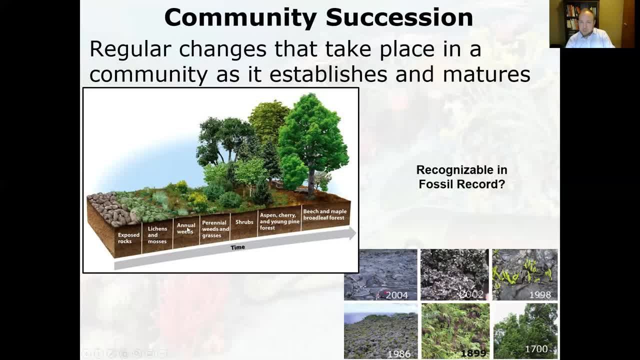 sort of moving in. first, Then we move up into annual weeds, sort of perennial weeds and grasses, Then we up into shrubs, sort of young pine forest, scrubby pine forest, And then into like a very mature kind of broadleaf forest. 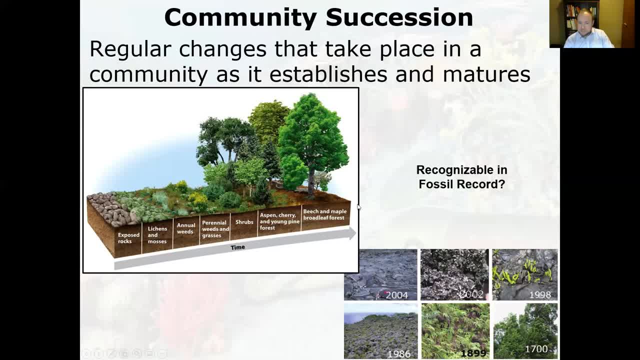 So this is a very well-established progression. We're able to see this, And it's actually even a way that we can sort of even date these events with this progression. So this down here is an example of a lava flow in Reunion Island. 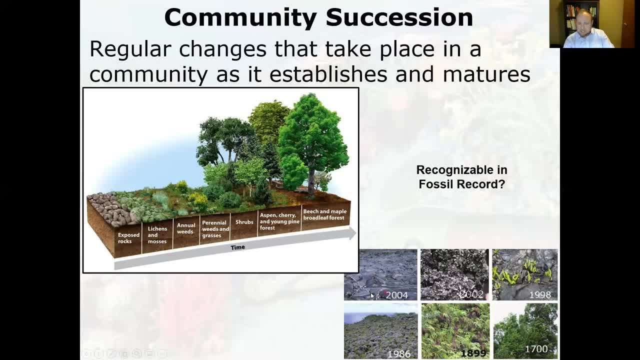 This is the lava flow that happened in 2004.. I'm not exactly sure what this picture was, but it's probably shortly after 2004.. You can see that the surface is pretty barren. There's not a lot going on. There are some things starting to populate in the cracks. 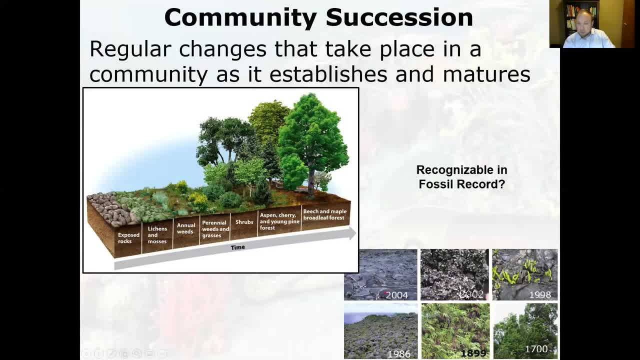 In 2000,. a lava flow that happened in 2002, slightly older. that lava flow surface is a little bit more weathered, a little bit more degraded And you see that these lichens and mosses and ferns are starting to populate the surface a little bit. 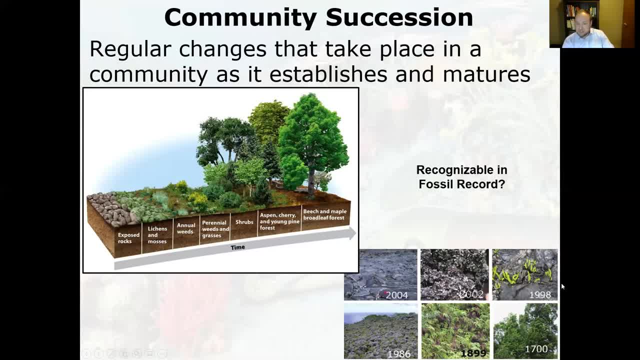 A lava flow in 1998, a little bit older than that. even we're starting to get sort of these grasses and weeds- One that happened in 1986, even older. the whole surface is starting to be kind of populated here something. 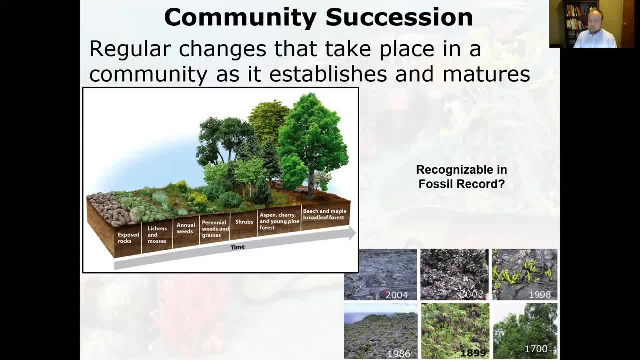 that is about 100 years old, sort of almost progressing to the shrub stage or the young pine forest, And then something that's about 300 years old has gone all the way through to the full-on forest stage. So we can actually use this well-established progression. 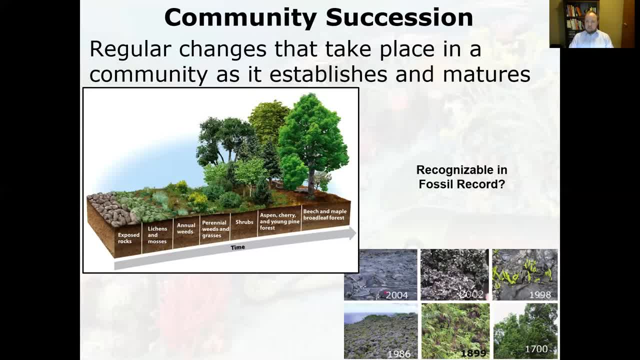 to date geologic features. Young lava flow is going to have a barren rocky surface with essentially no plant life, And an older lava flow might be severely degraded and actually hosting Now a full-on forest environment. So thinking about these timescales here, 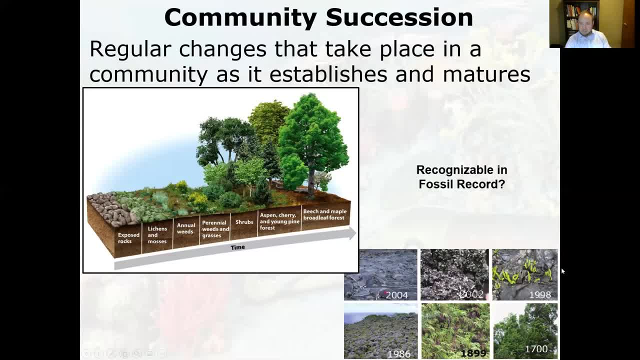 progressing here in like year, maybe like decade, decade century, a couple centuries. do you think that this progression, this succession, would be recognizable in the fossil record? So think about the sedimentary record, Think about bedding, Think about how much time an individual 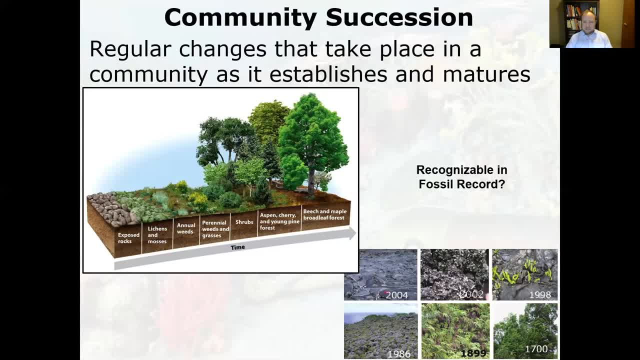 bed represents. Do you think that we're able to see this? Probably not. So a lot of studies sort of start attributing changes in the ecology to this idea of succession, But succession probably happens too quickly. We're probably not able to actually see that. 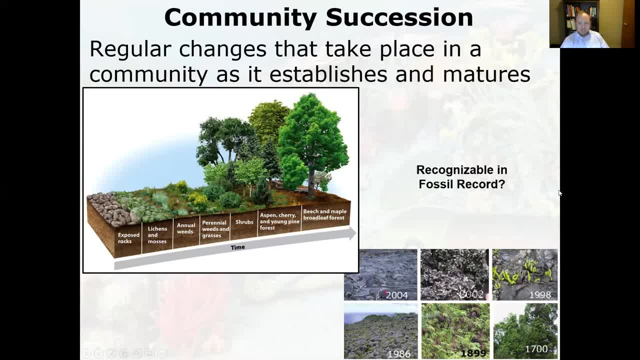 in the fossil record. So think about not only just the preservation biases, but also the time biases. Unfortunately, reading the fossil record, reading the rock record, It's like reading a novel with a bunch of the pages ripped out. We're missing time. 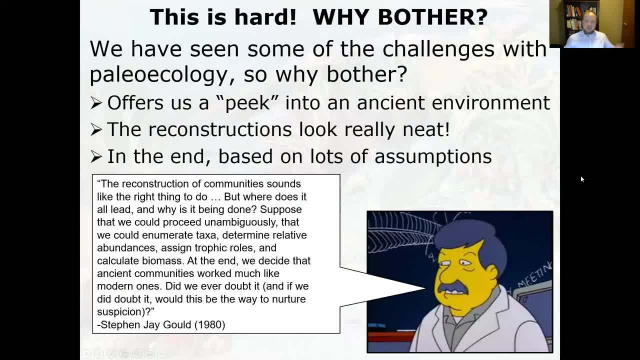 We're missing things. So this is really hard. Why should we bother? Why would we do this? We've seen a lot of the challenges that it offers. Why bother? Well, it's really neat to get a little peek at an ancient environment. 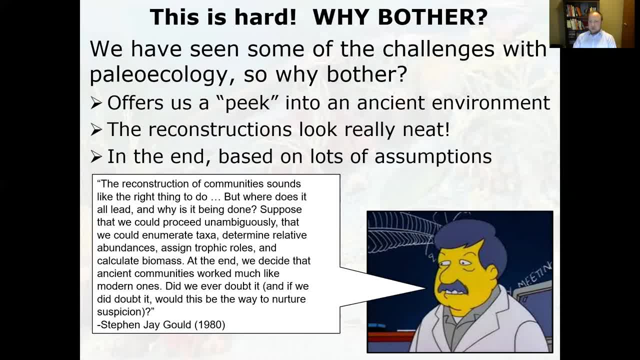 What was life like in the Ordovician? So, thinking about rocks around here going to an exposure, you're the first one that's seen that exposure. in some cases, Light has not shined on those rocks in hundreds of millions of years. What was that like when it was actually? 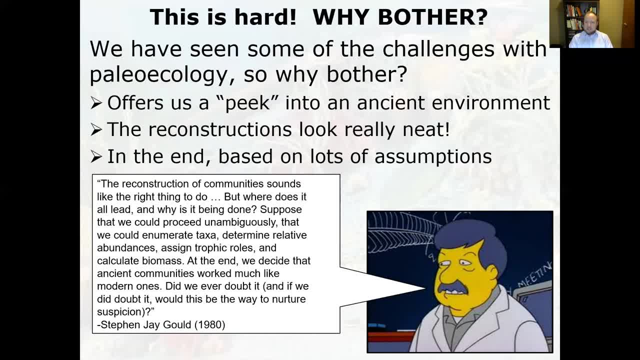 a thriving living community. What was going on? Who was eating who? Who was digging around, Who was swimming around? What did it look like? So when we put this all together and we make these reconstructions, they look cool. They're neat. 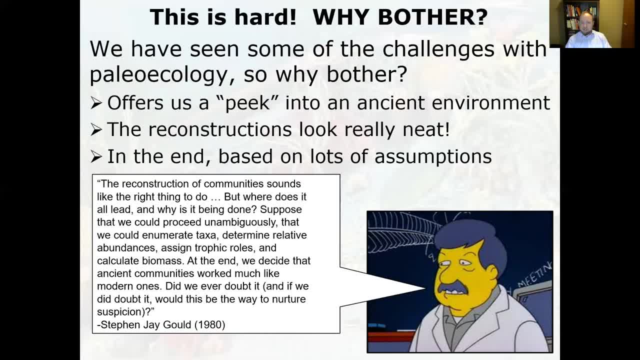 I like looking at all those artistic renderings of what life was like, But we need to remember that in the end it's based on a lot of assumptions, In a lot of cases, some very valid assumptions, very safe assumptions In a lot of cases. in other cases maybe not. 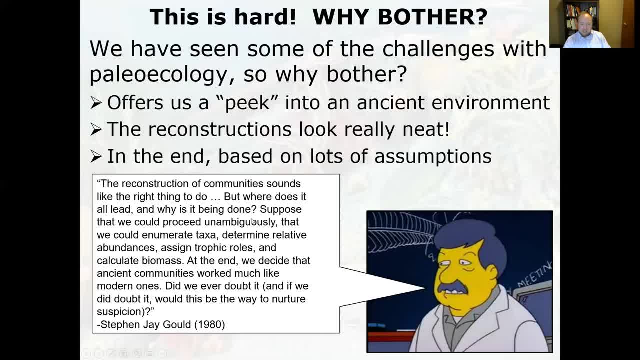 So Stephen Jay Gould has this quote here: Reconstruction community sounds like the right thing to do, but where does it all lead and why is it being done? Suppose that we could proceed unambiguously Now. remember that's a trip right. 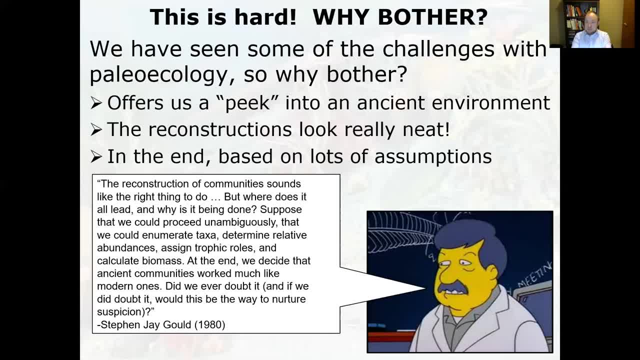 So figuring out the entire living, living, living, living, living assemblage unambiguously. figuring out the environment unambiguously. We could then enumerate taxa. We could see every creature that was living there, every organism, determine the relative abundance. 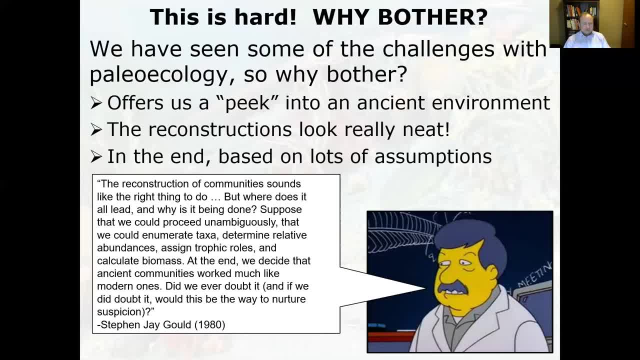 assign all their trophic roles on the food pyramid and calculate their biomass. Let's say that we could do that And again, we've talked this whole lecture about all the challenges with that. At the end we probably decide that ancient communities worked. 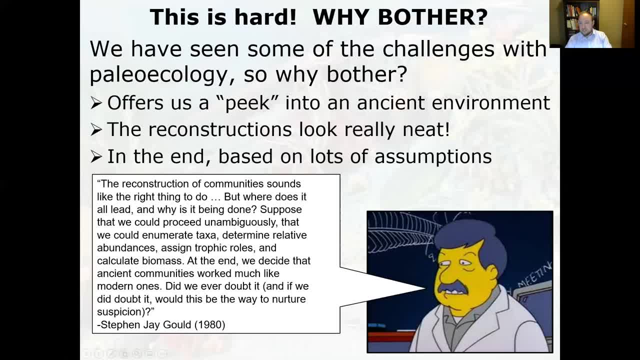 much like modern ones. Does that help us at all? Did we ever really doubt that? Again, one of the key things in geology: uniformitarianism. the present's the key to the past. OK, ancient communities worked the same way. 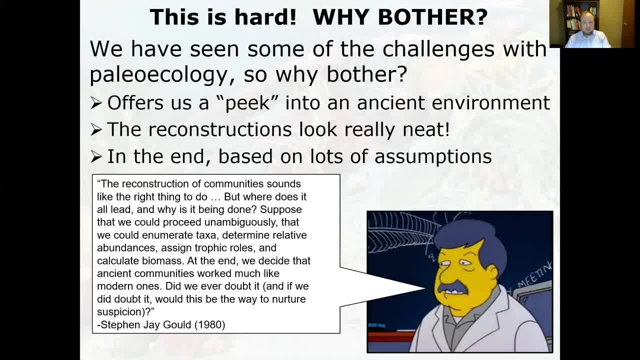 that modern ones do. probably Essentially, our reconstructions of ancient communities are based on that assumption. So of course that's what we're going to think. So maybe we can do that. Maybe we can do that, Maybe we shouldn't really be doing that all that much. 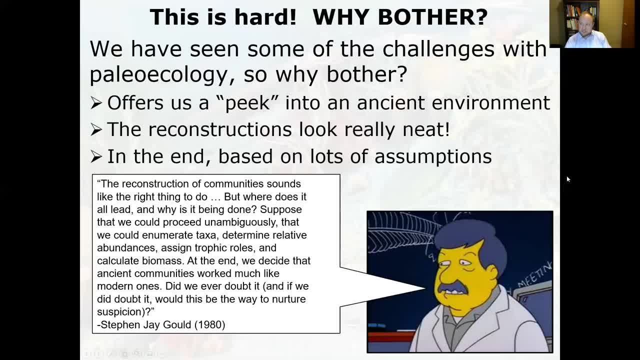 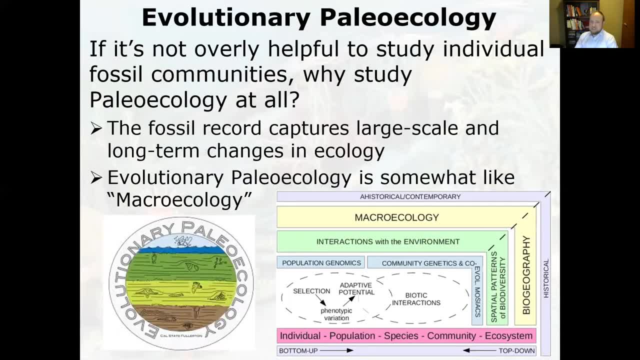 Maybe we shouldn't be focusing so much on reconstructing environments for the sake of reconstructing environments. Next class we're going to talk about evolutionary paleoecology, So if it's not helpful to do that, why study it at all?